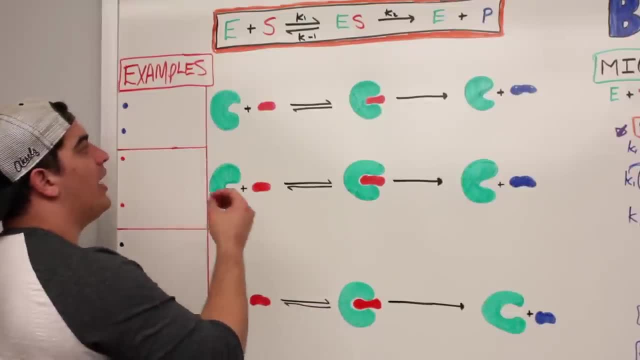 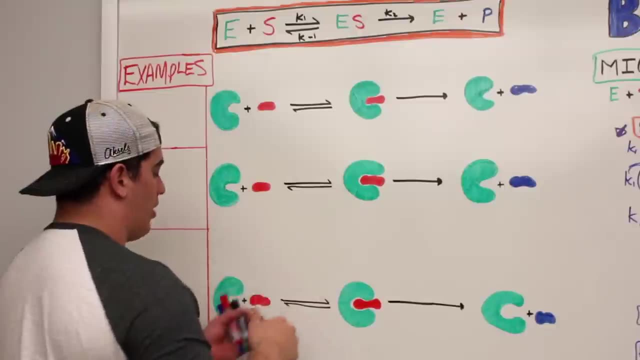 of a conceptual matter to under, to explain something called inhibition. So if you look here in green, I have my enzyme, In red I have my substrate, I have my double arrows. And again, what would this one be? This would be K1.. This would be K-1.. And this would be. 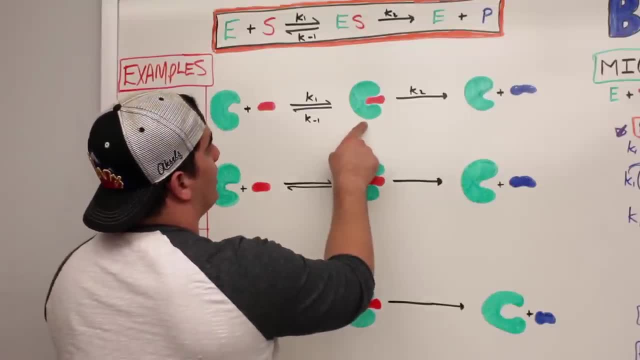 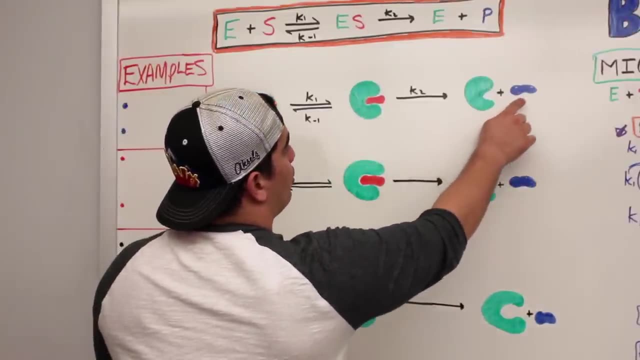 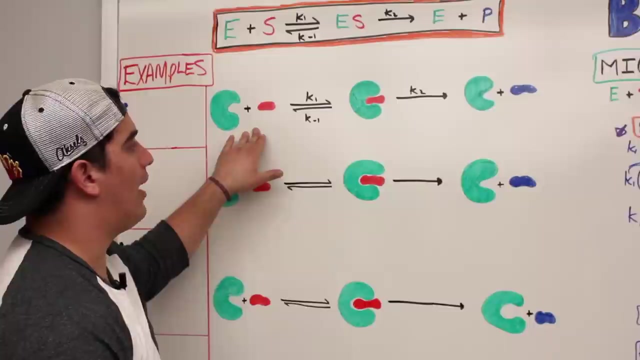 K2.. This green right here is the enzyme, The red right there is the substrate. So this whole thing is the enzyme substrate. This green right here is the enzyme And this blue structure right there is the product. What we're going to do in this video is we're going to talk specifically about how inhibitors 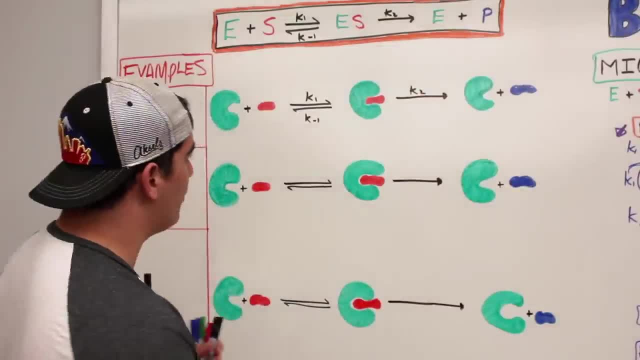 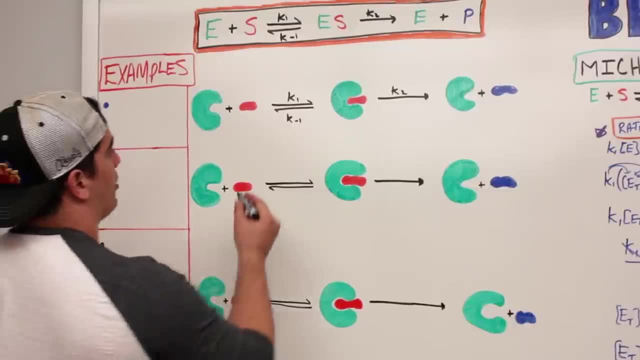 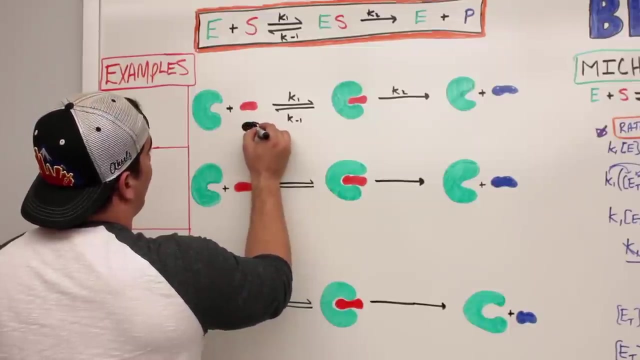 can affect this normal process. So in the first one we're going to talk about what's called competitive inhibition. So what happens in competitive inhibition? Let's say, right here I draw in black. Let's say that I want to look at a competitive inhibitor. Now, a competitive inhibitor is: 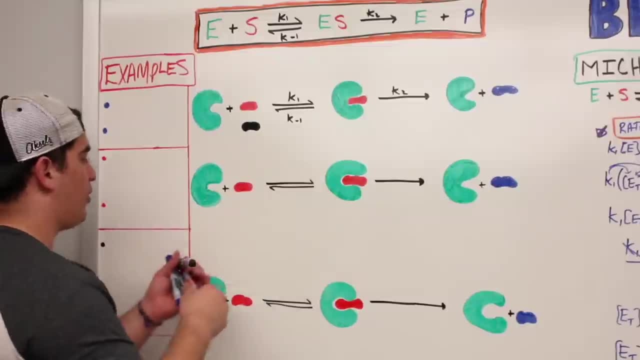 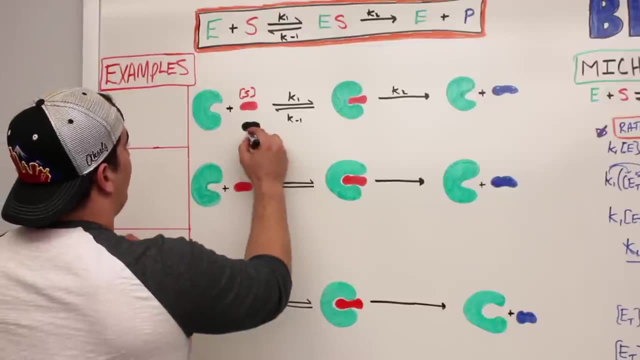 structurally similar to the normal substrate. So here in the red is our substrate. I'll put substrate above that And here in black is going to be our competitive inhibitor. If you look, their structures appear almost exactly similar. What happens in this reaction? 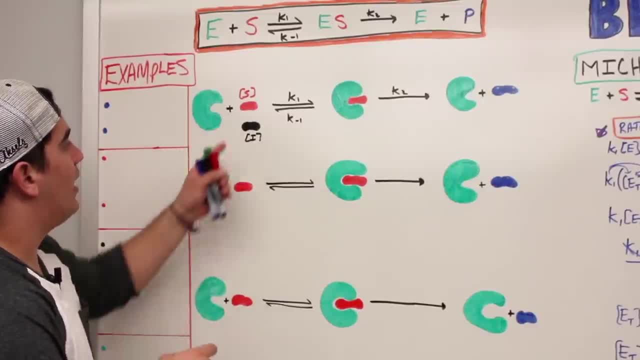 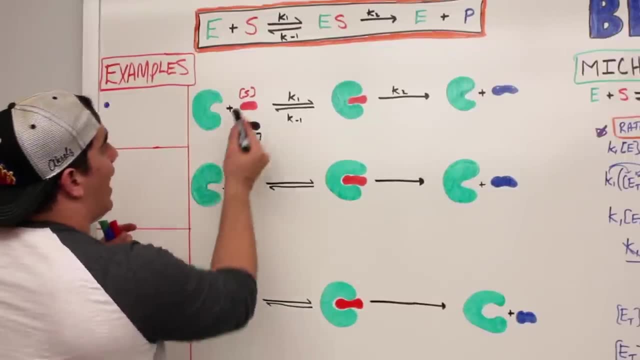 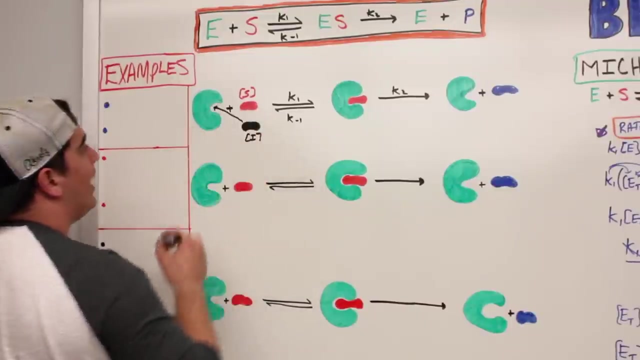 is, as the substrate is trying to react with the enzyme, the inhibitor might have more affinity for the enzyme. Okay, The enzyme might have more affinity for the inhibitor than the substrate. And so, for example, what will happen is the inhibitor will come in here and bind into the active 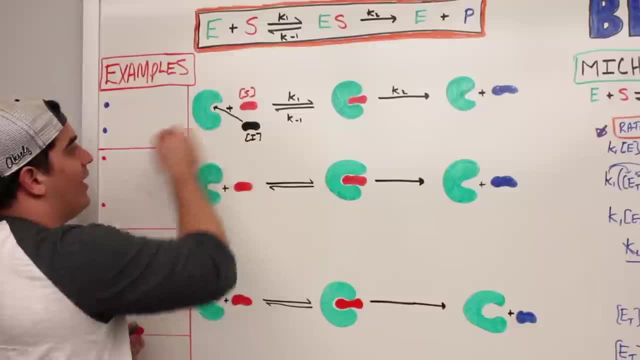 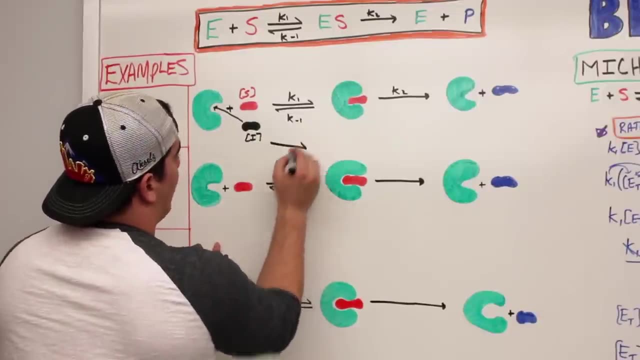 site of this enzyme And then look what happens. Can the substrate get in there if the inhibitor is bound? No, So then what does it look like afterwards if I were to draw the product of this reaction here? Let's say, I have one arrow going this way and this is a reversible reaction. 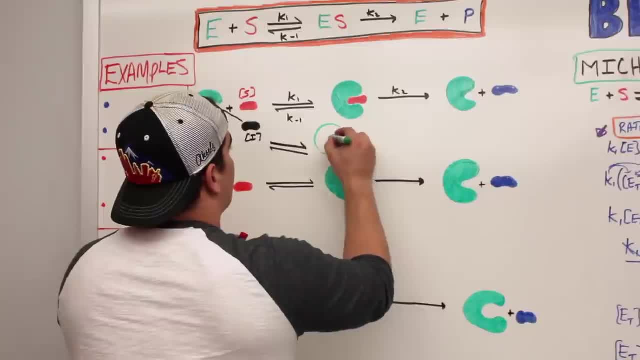 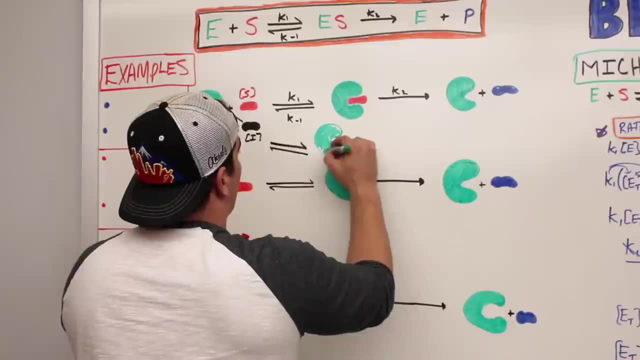 What would it look like? I would have something like this. So now I would have my… So I would have my enzyme here And again. what's going to be bound to the active site of this enzyme? It's going to be an inhibitor, And when the inhibitor binds…. 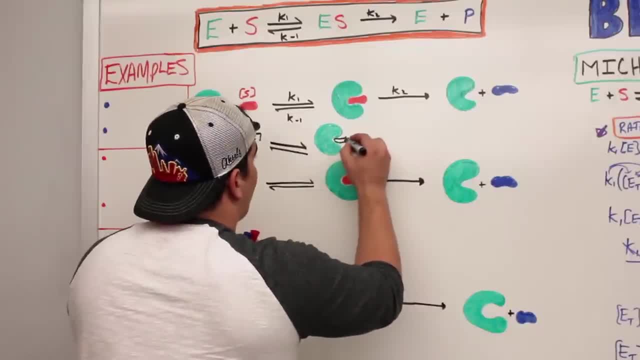 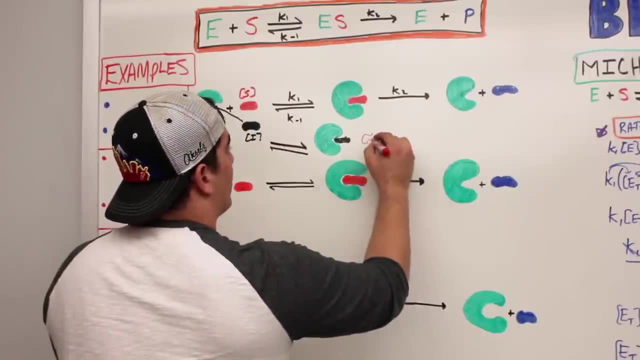 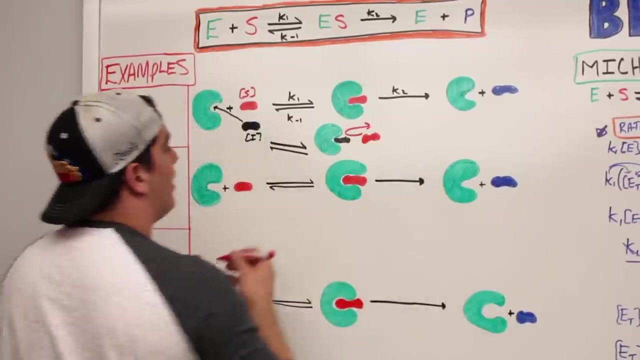 So now let's draw the inhibitor fitting into that active site pocket. Now what can't happen? The substrate can't bind. So let's draw the substrate over here. The substrate, it can't bind into that active site. So because the substrate can't bind into the active site, 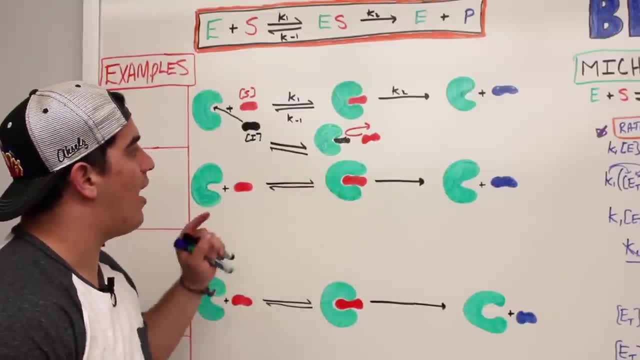 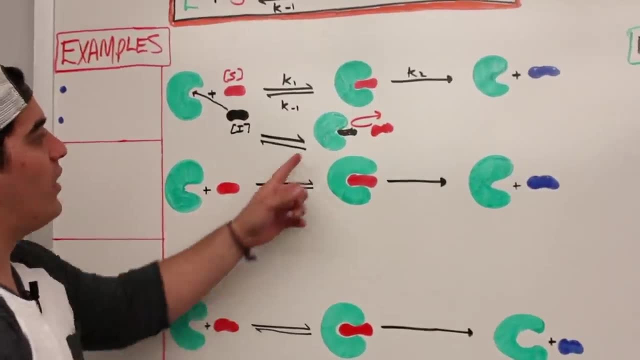 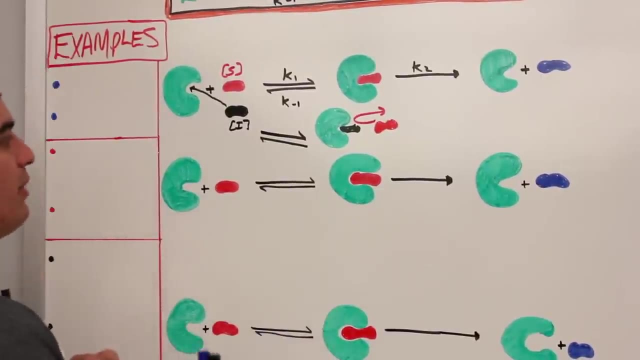 the enzyme's affinity for the substrate goes down and its affinity for the inhibitor goes up. Now, the only way that this reaction can continue to proceed is if you do something. So, if you think about this, let's think about what's called Le Chatelier's Principle. 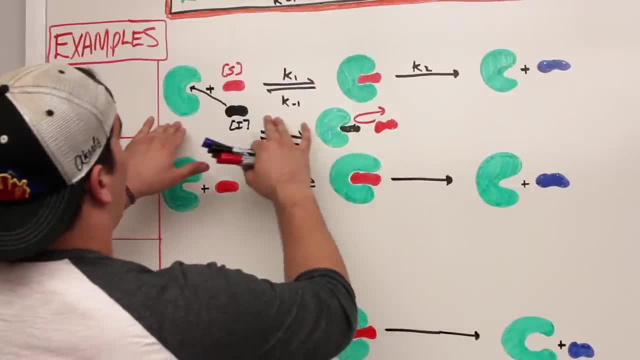 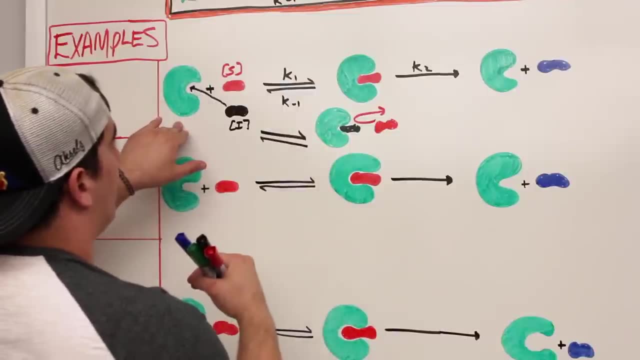 So Le Chatelier's Principle says: in this case, what's happening here to the formation of my enzyme substrate? Well, if the inhibitor is binding there to the enzyme, I'm not taking as much enzyme substrate, right? So my enzyme substrate concentration isn't. 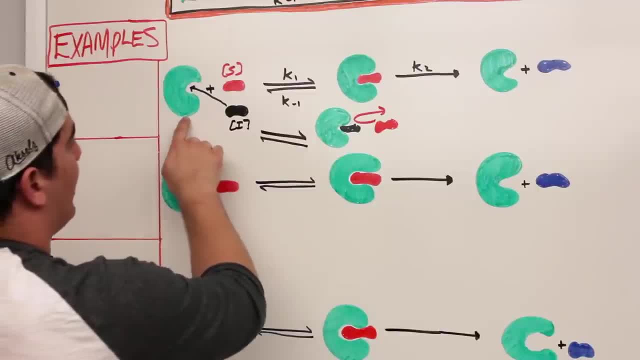 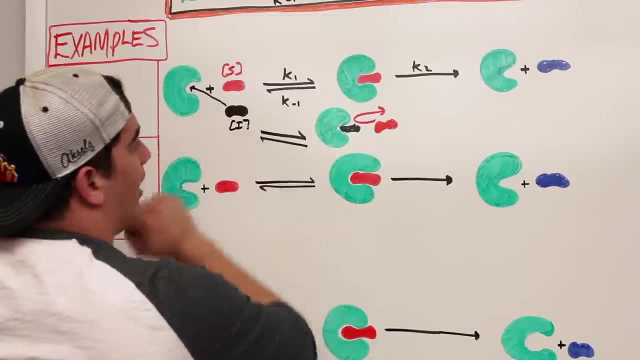 really going up. But if you think about this with my enzyme, the enzyme is binding a lot to this inhibitor, right? If it's binding a lot to this inhibitor, it's not binding with the substrate. So if you think about this, let's think about like a seesaw. 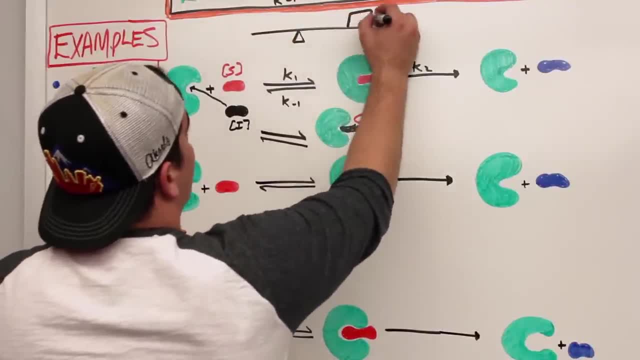 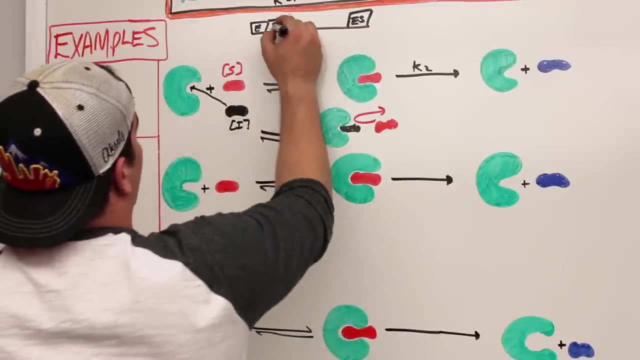 here. So let's say, here I have a seesaw. Let's say, on one end I have the enzyme substrate, and let's say, over here, on this end I have the enzyme and we also have the substrate. In this case I'm not making enough enzyme substrate. 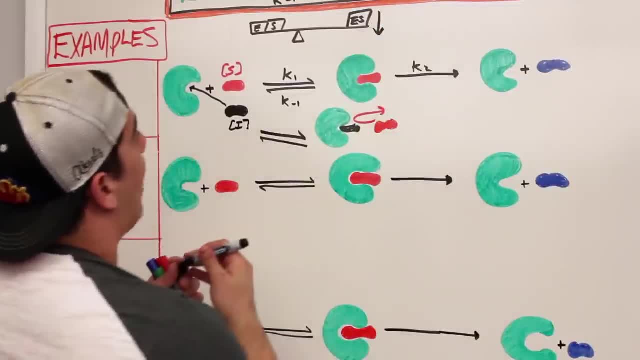 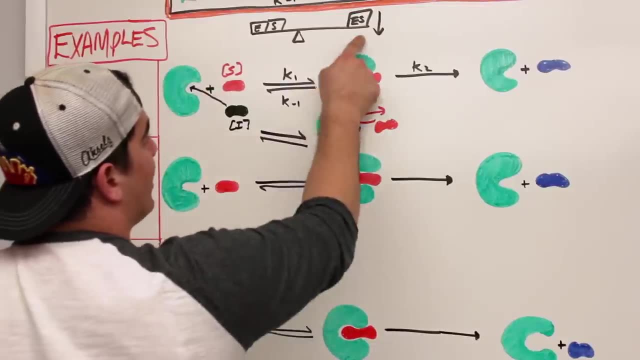 So what's happening to this? This, like you can think about this as going down, right. Now the amount of enzyme that's reacting with the substrate also is decreasing, right. So again, this is going to decrease. Now Le Chatelier's principle says: 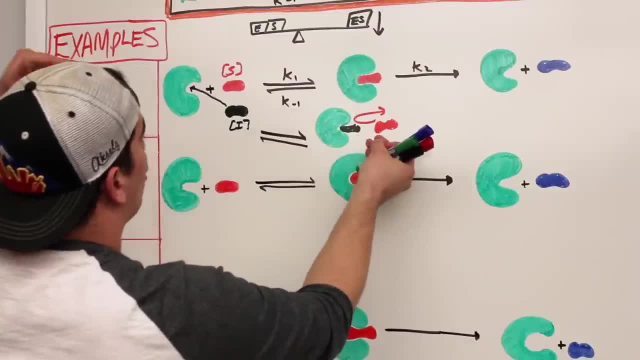 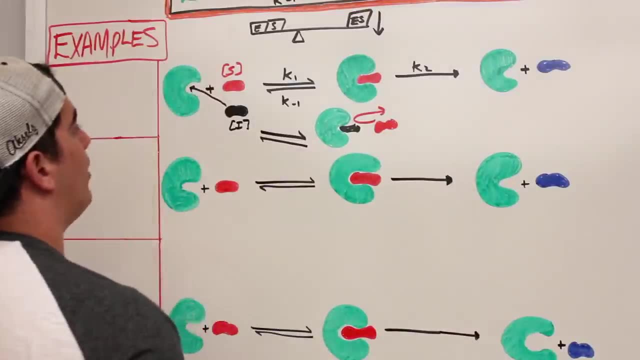 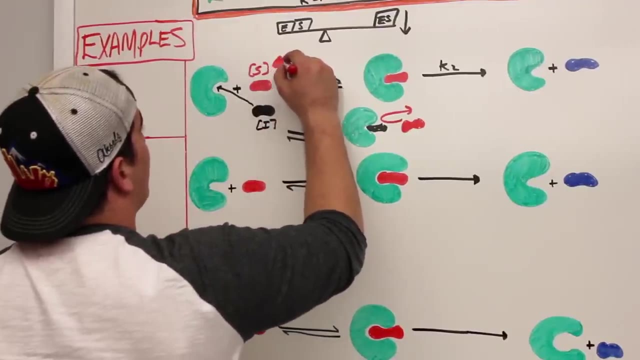 that whenever this side of the equation is decreasing, you're going to want to shift the reaction to the right to increase the concentration of the enzyme substrate. Well, how do I do that? By increasing the substrate concentration. So if I increase the substrate concentration enough, 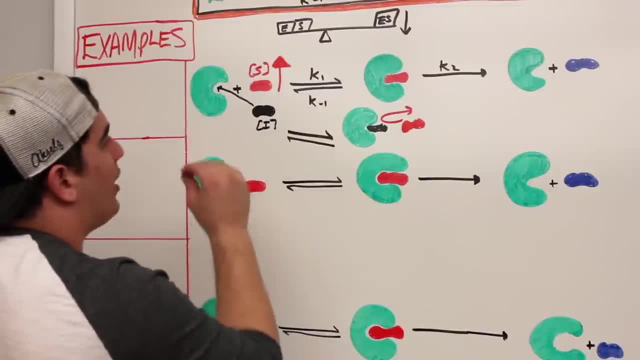 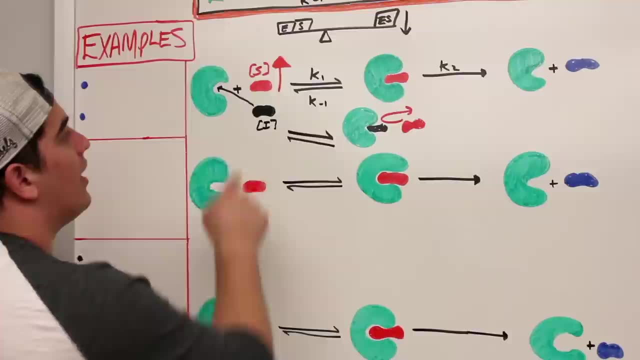 to where the affinity that the enzyme has for the inhibitor might go down a little bit and the substrate might compete and out beat the inhibitor to that active site. then what can happen? Then I can form more enzyme substrate. So again one more time with competitive inhibitors. 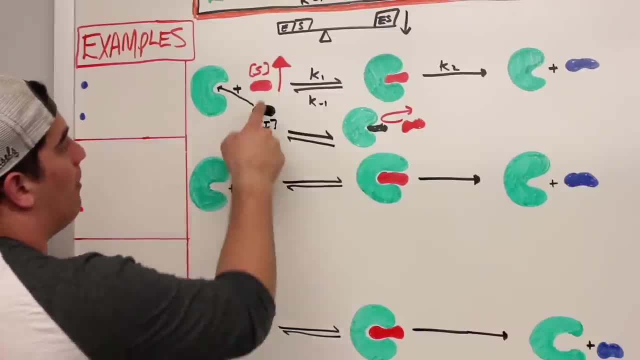 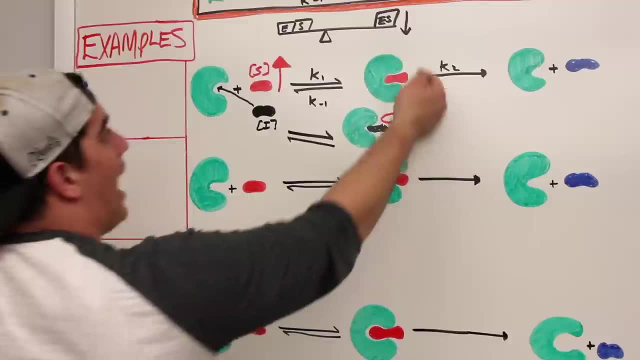 Competitive inhibitor will bind onto the active site of this enzyme, block the substrate from binding. So now you have this structure here, The only way that I can form more enzyme substrate. because what's happening? according to Le Chatelier's principle, the amount of enzyme substrate that I'm making is decreasing. 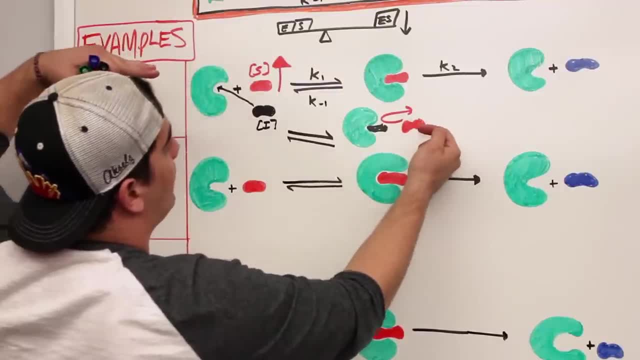 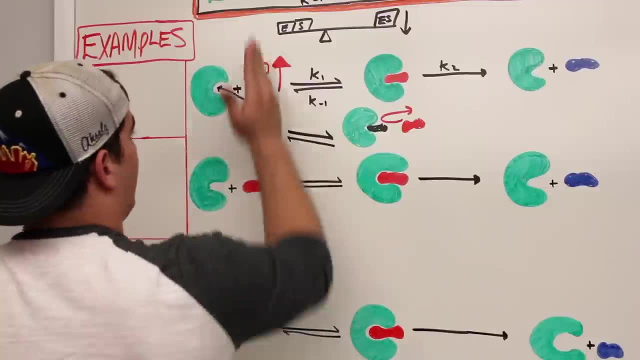 If the amount that I'm making is decreasing, Le Chatelier's principle says I have to shift this reaction to the right to increase the concentration of my enzyme substrate. So what do I have to do? I need to increase the amount of substrate. 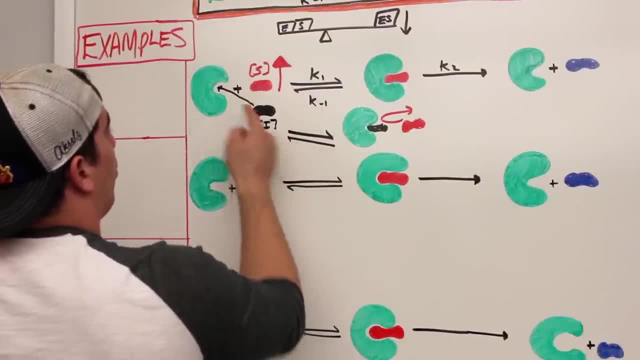 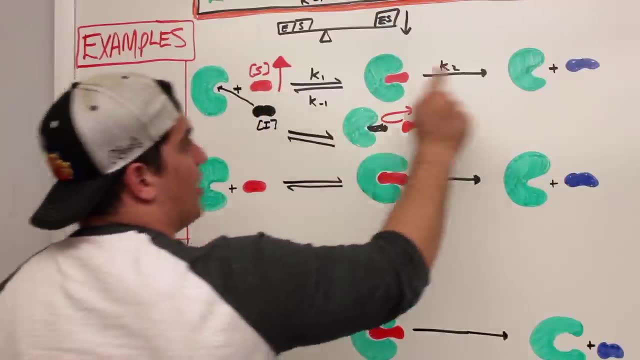 If I increase the amount of substrate, less of the inhibitor, more of the inhibitor will bind to the active site and more of the substrate will bind to the active site and form our enzyme substrate complex, which will disassociate into enzyme and product. So again, what is this one right here called? 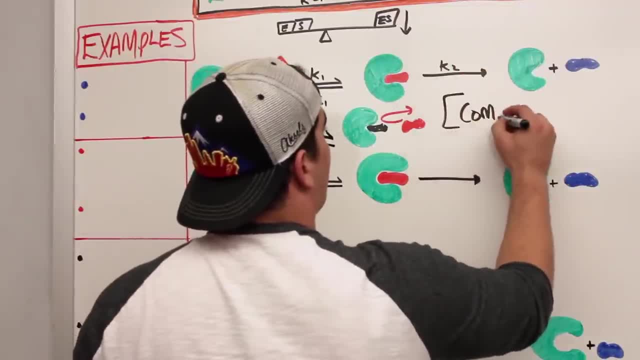 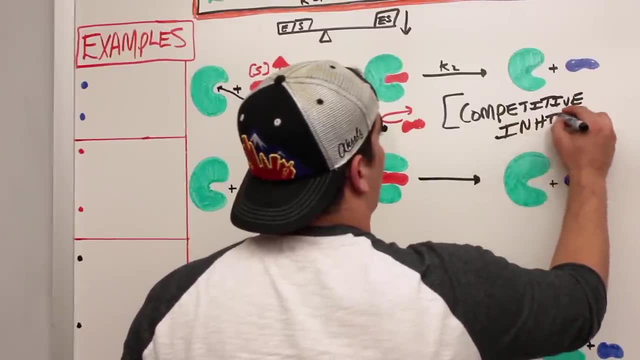 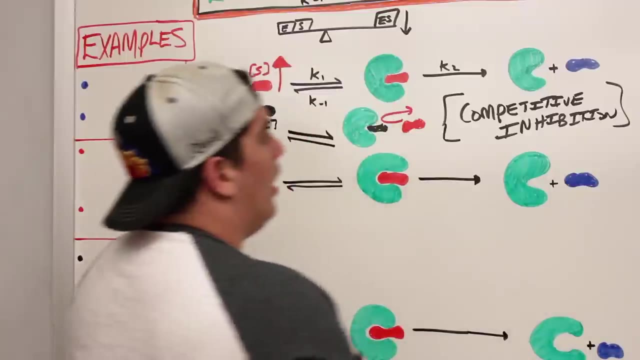 This one is competitive inhibition And this one is super, super important. All of these are super important. This one's of the most common usually. But if we think about it, what could we do? as, because you know, there's normal inhibitors, all. 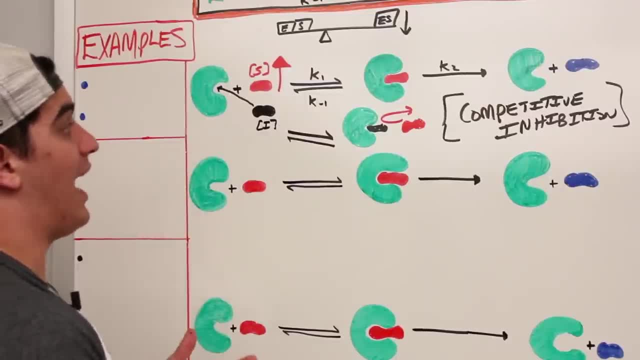 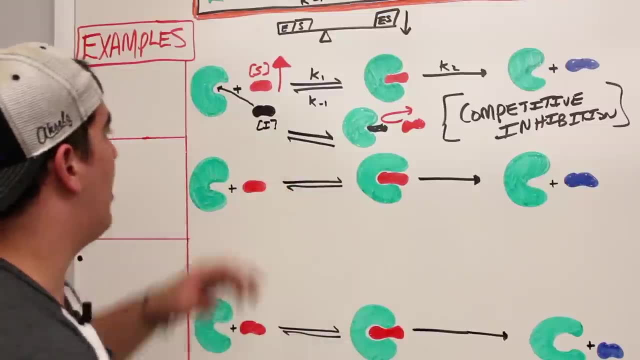 around in everything that we do, We can actually think of drugs. actually, that could act as competitive inhibitors. That could actually be a good thing. So, for example, what would be a normal example of a competitive inhibitor that would inhibit a specific enzyme, maybe in our body? 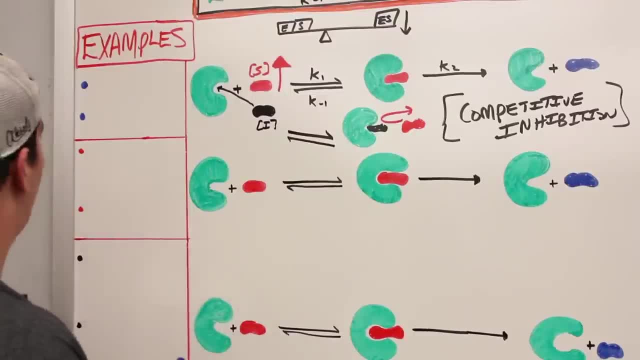 So, for example, we could say statins. So statins, Statins are basically, they're trying to lower our normal cholesterol levels, so they're good for hyperlipidemia and hypercholesterolemia. What does statin do? 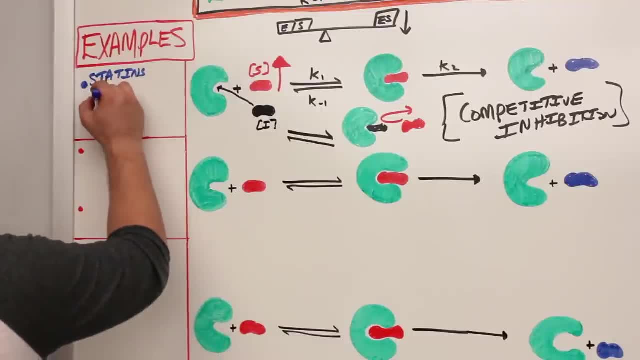 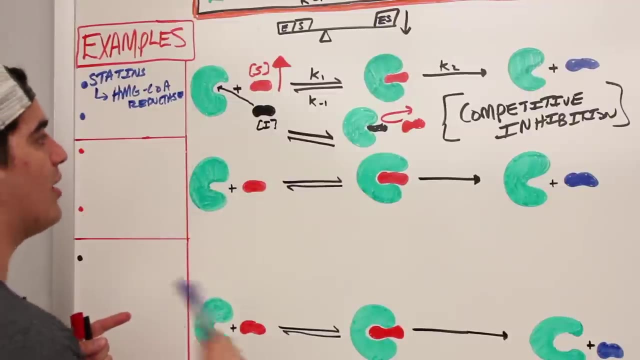 Statin actually binds on to the active site of a specific enzyme that regulates cholesterol synthesis and that's called HMG-CoA reductase. So we're just giving you some real life applications of competitive inhibitors. And what is the whole concept? An inhibitor's binding on to the active site of a specific 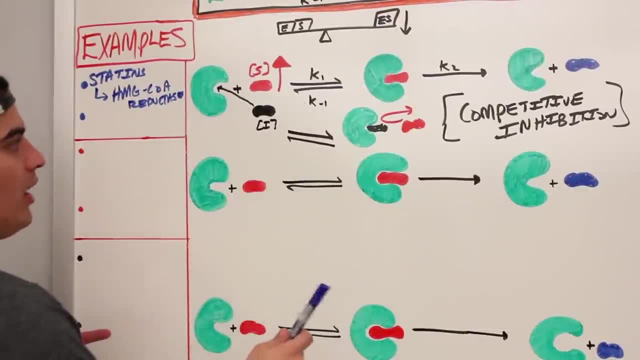 enzyme blocking the substrate from binding. But if you increase the substrate concentration you can overcome the amount of inhibitor that's binding and form more enzyme substrate. And we're going to talk about KM in just a second. with this one, Another example, I'll just give you another one. 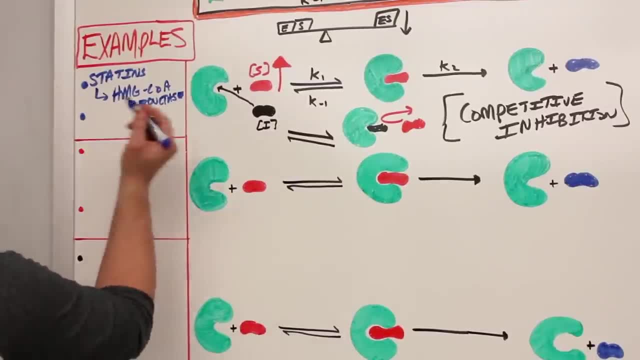 High blood pressure. So they actually use another drug here It's called ACE inhibitors, like captopril, enalapril, losonopril. So ACE inhibitors bind to the active site of ACE enzymes, So it actually inhibits. 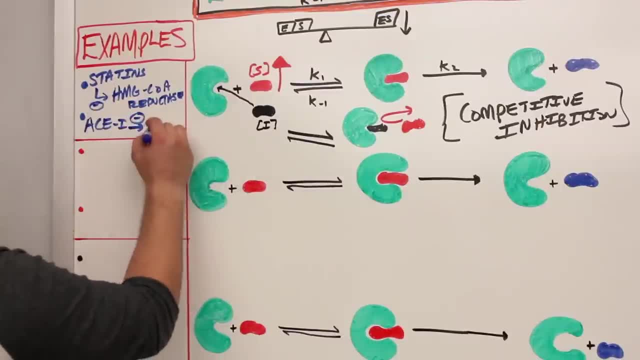 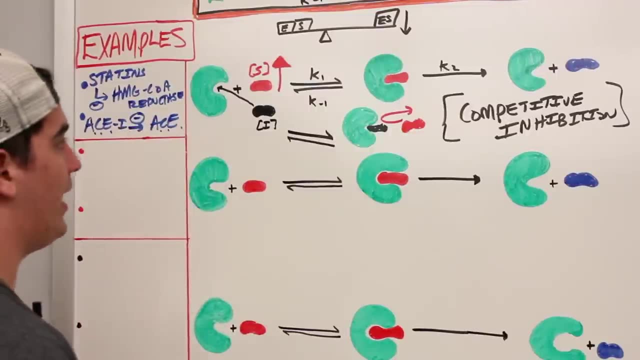 So statins inhibits HMG-CoA, HMG-CoA reductase, ACE inhibitors would inhibit ACE, which stands for angiotensin converting enzyme. So just some practical applications of competitive inhibition. Now one more thing I want to mention. 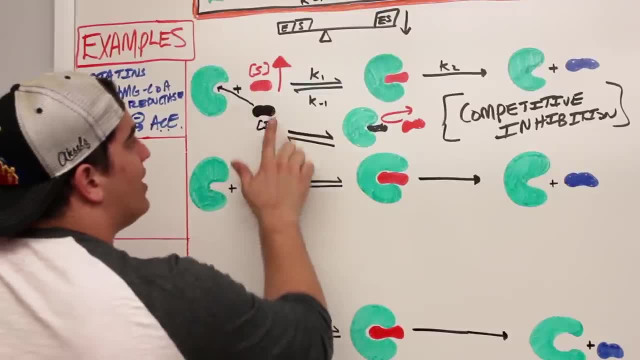 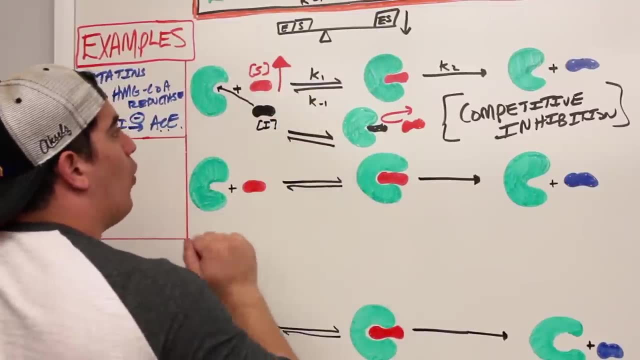 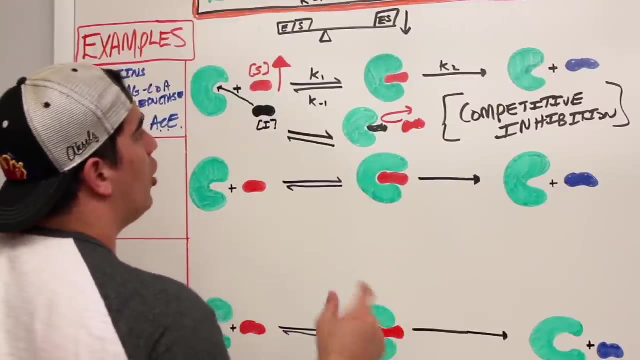 about competitive inhibition. What did we have to do to get this enzyme and substrate to form more enzyme substrate? We had to increase the substrate concentration. Well, remember we said KM is equal to the substrate concentration, right with respect to half the Vmax. 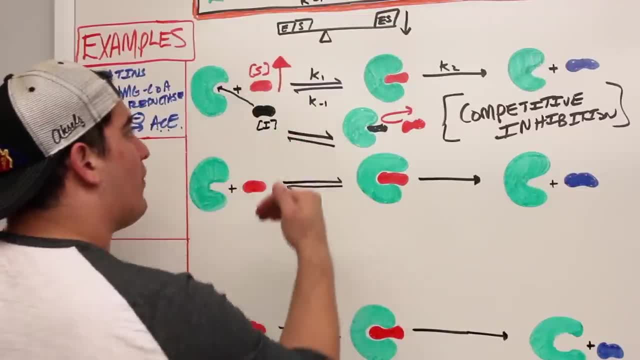 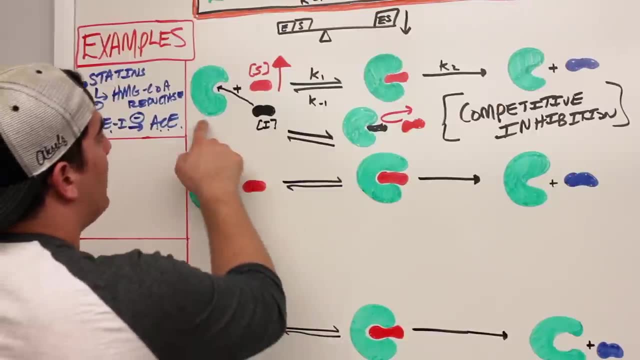 Well, what I did was I increased the substrate concentration, So I threw off the normal equilibrium with this reaction. So now what I have to do to account for this increasing substrate concentration is the KM, because there's more substrate. what did I say? 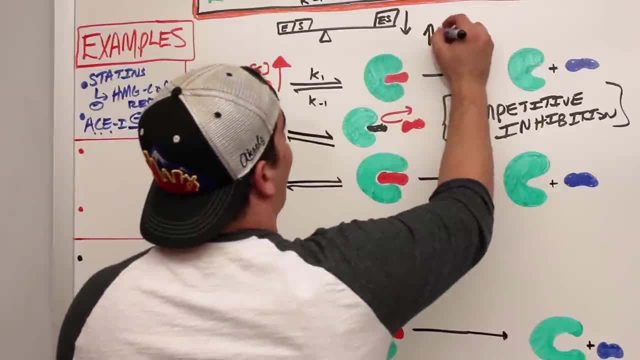 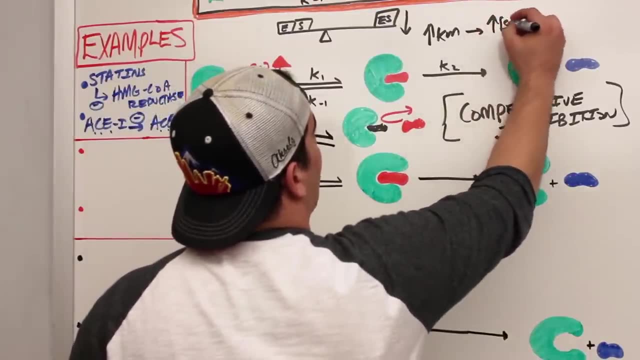 Remember that relationship. I said That with increasing KM, the enzyme will have to take on more substrate. So if there's an increase in KM, it's because there was a increase in substrate concentration. So what's happening? What's happening to the KM, or you? 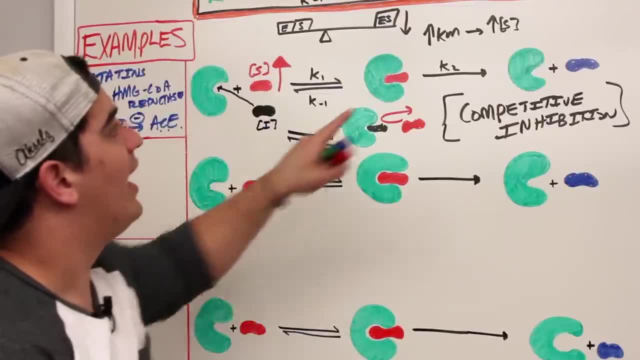 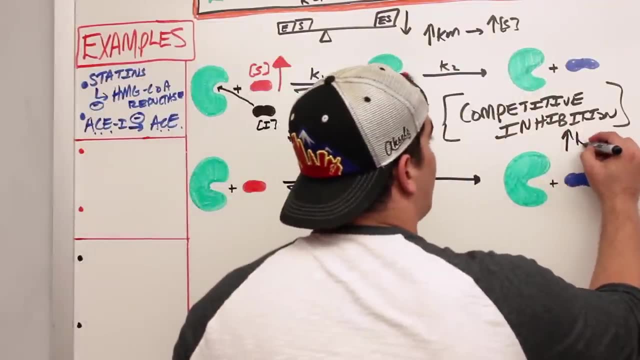 can say the affinity that this enzyme has for the substrate. It's increasing because we have to increase the substrate concentration. Super, super important here, So competitive. we increase the KM, But did we affect the amount of product that's being formed? 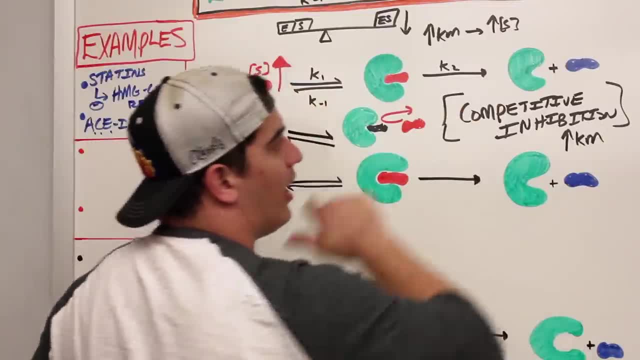 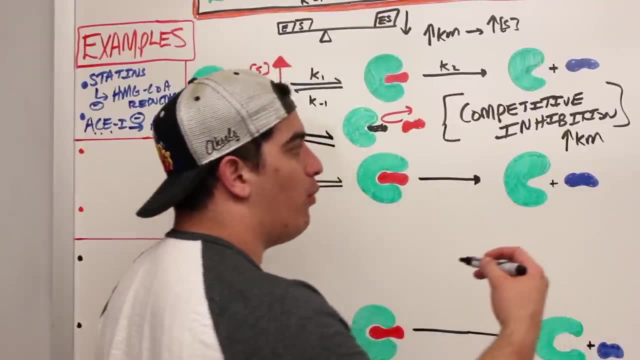 No, because we increased the substrate concentration. so we're still going to make our normal amount of products. So Vmax, which is the maximum velocity- the saturation point to where the enzyme can be no more saturated- still occurs, So we can still reach Vmax. 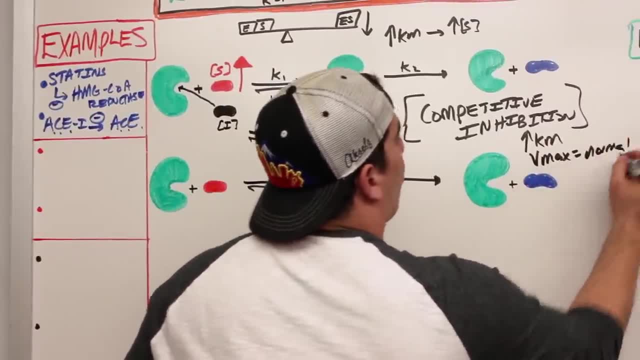 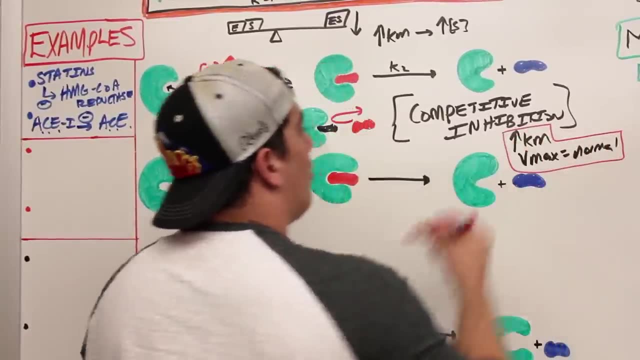 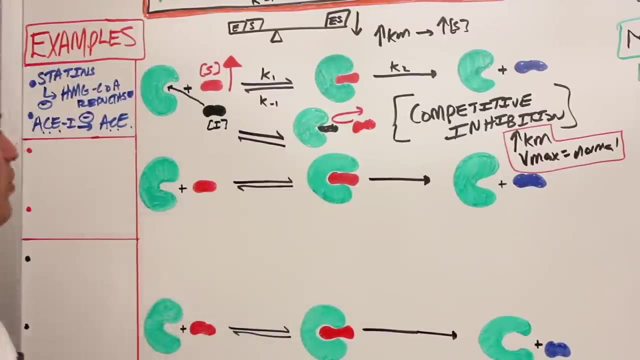 So we'll say Vmax is normal or unchanged. OK, These are two big concepts that I need you guys to grasp from this inhibition. OK, so that covers competitive inhibition. Let's move on to the next one. So the next one that we're going to do is: 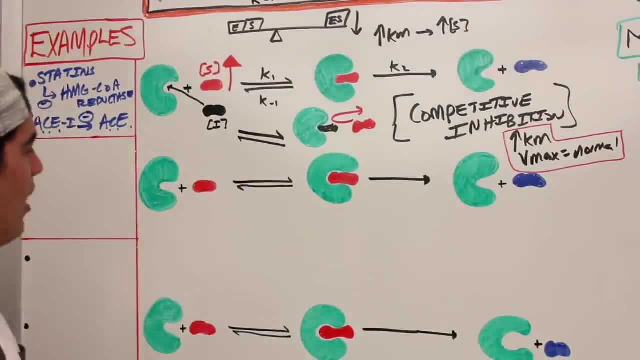 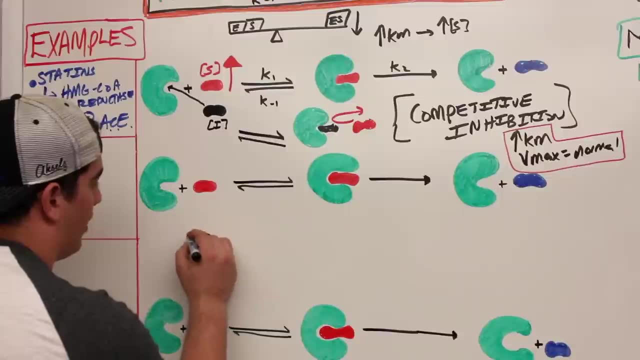 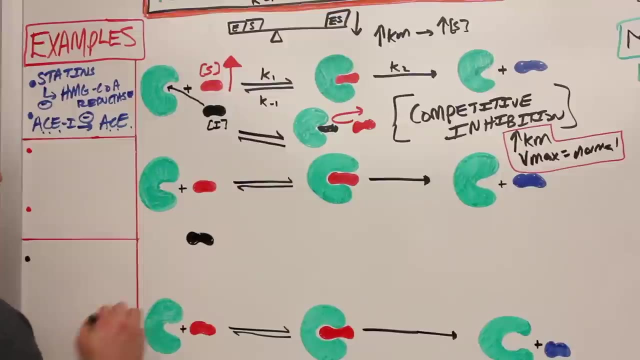 let's talk about non-competitive inhibition And non-competitive inhibition. it's a little different. Now. non-competitive inhibition, let's say again: I draw here in black, This is my inhibitor, But what happens is the inhibitor doesn't bind onto the active site. 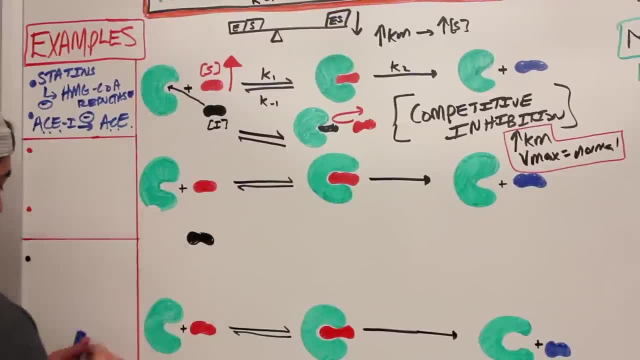 There's a little pocket here on the enzyme. There's a little pocket that's kind of always open here on the enzyme And what happens is this inhibitor right here. so again, what's this guy right there? This is my substrate. 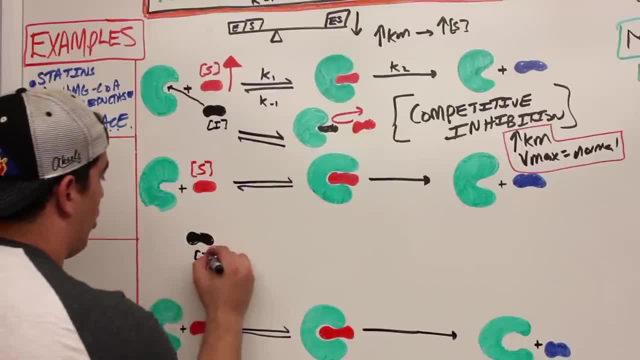 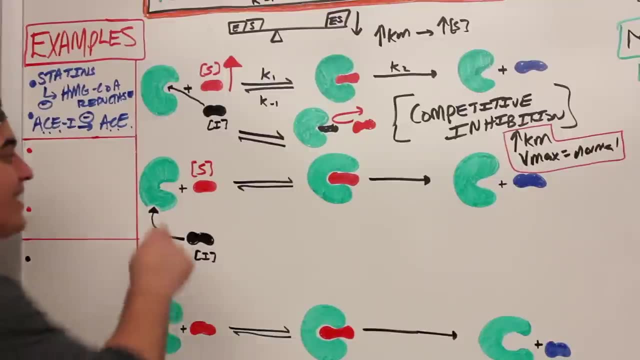 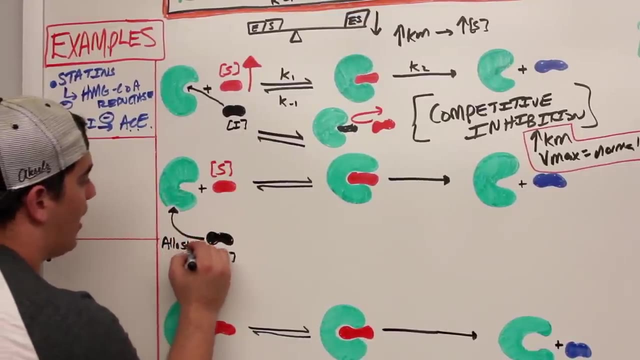 And then what's this black guy right there? This is our inhibitor. What can happen is this inhibitor can actually come on and bind to this other site of the enzyme. That's not the active site. That site right there is called the allosteric site. 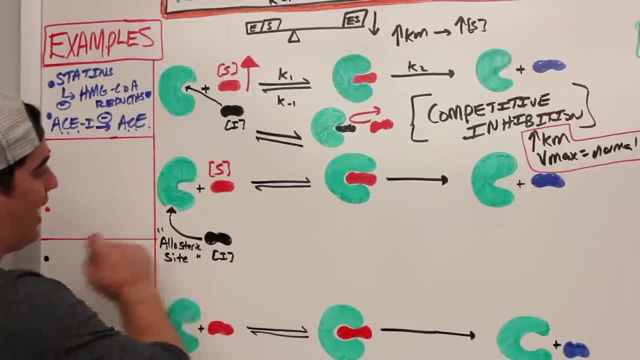 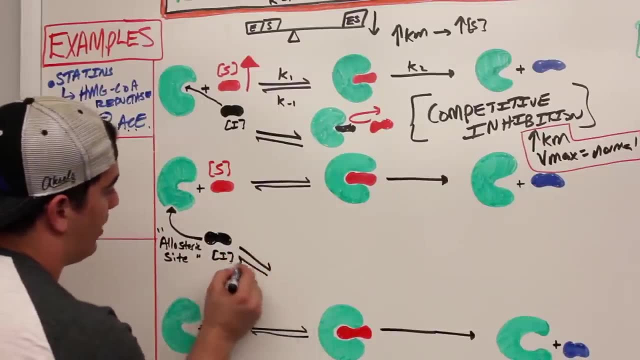 OK, And what happens is when the inhibitor comes in and it binds onto that free enzyme- remember, it's free enzyme. what do we get out of this? Let's see. I draw this double arrow because this can be reversible. I'm going to have something like this: 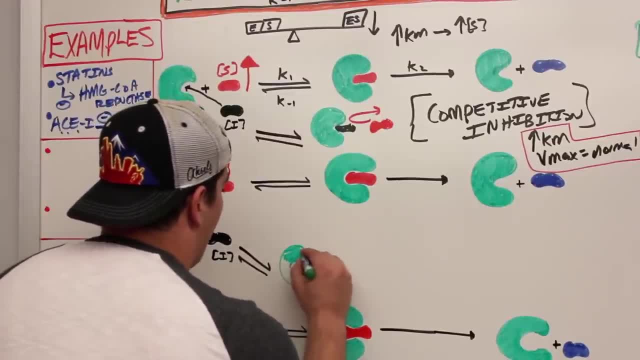 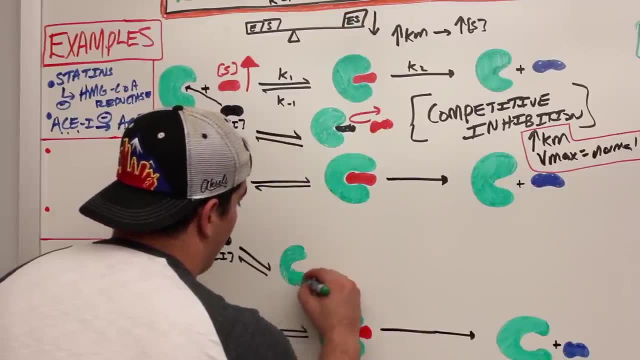 So I'll have my enzyme here And the inhibitor will. I mean, the enzyme will not be bound to the substrate because it's bound to the inhibitor, right? So if we look here, what will happen? It'll have this little pocket here, right? 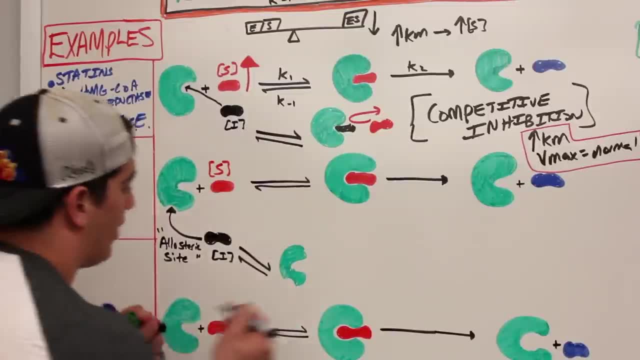 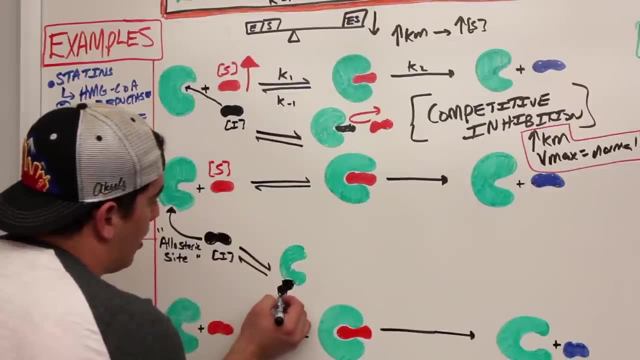 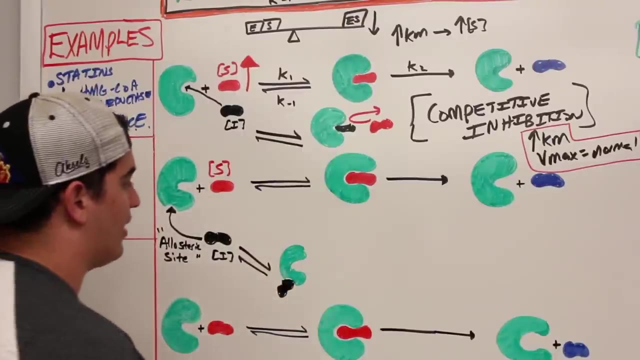 So I have this little pocket there. And then what happens? This inhibitor is bound onto that guy. But now look what happens here. This enzyme, This enzyme- can still react with substrate. It can still react with substrate. That's not going to stop this reaction. 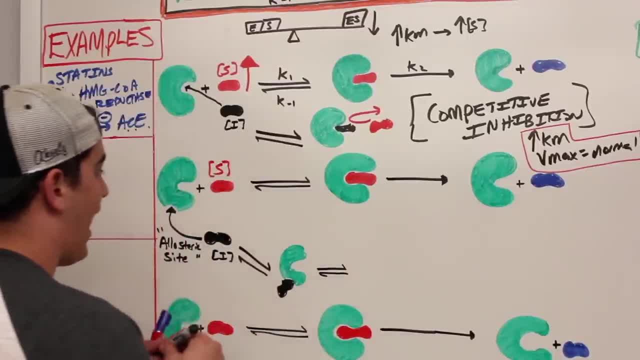 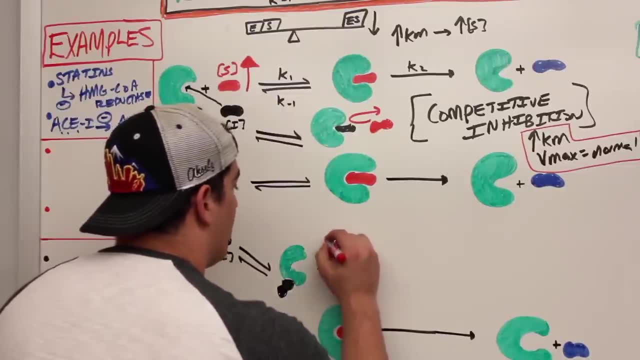 So if I go ahead in this reaction and I react this enzyme inhibitor right with my substrate- So let's say now I react it with my substrate- The substrate can still bind, It can still bind in there into that active site. 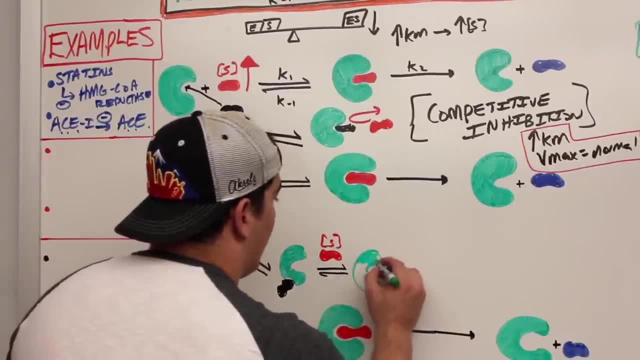 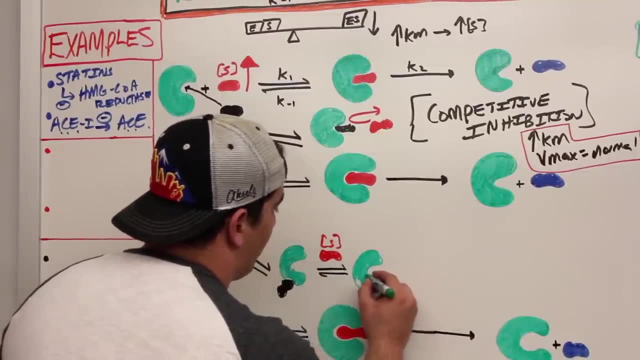 So now look what we have here. So now look what we got here. Something not good, right, Something not very good. It's a beautiful thing, but not necessarily good for this enzyme. So what happens here? So now look what we have here. 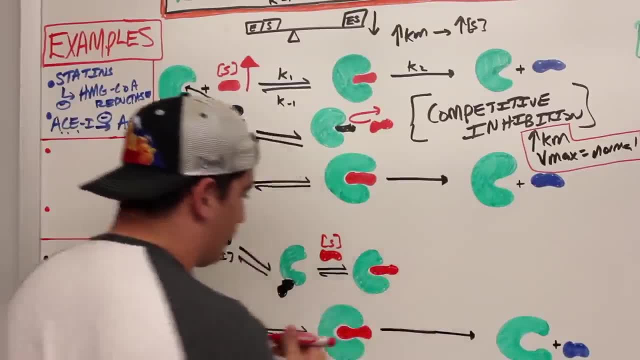 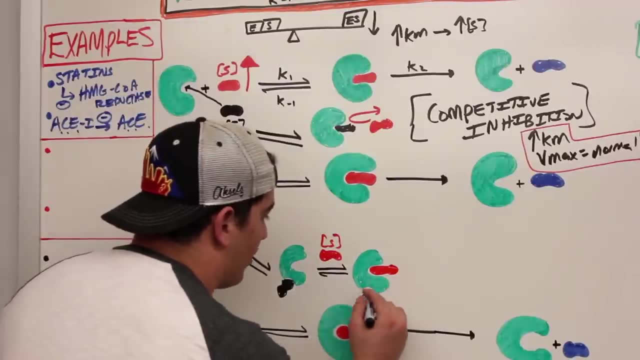 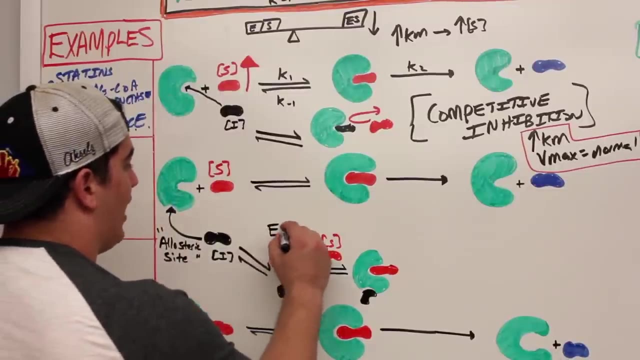 We'll have the substrate bound into the active site still, And the inhibitor is still bound in that little allosteric pocket right there. So it's still bound in that allosteric pocket. Now look what we have here. Here we had a enzyme inhibitor complex, right? 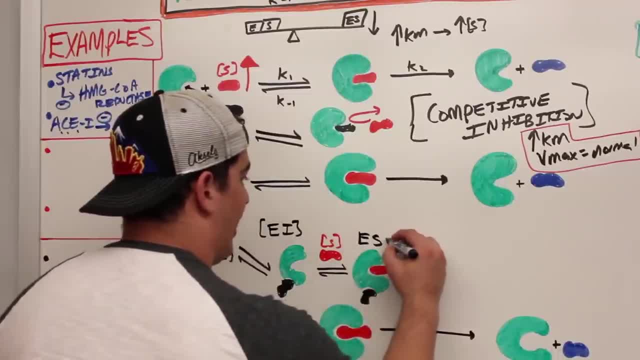 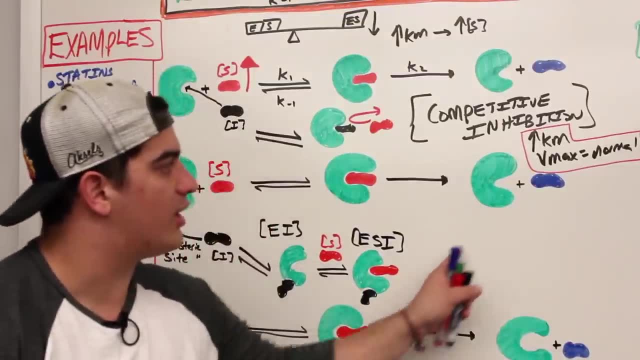 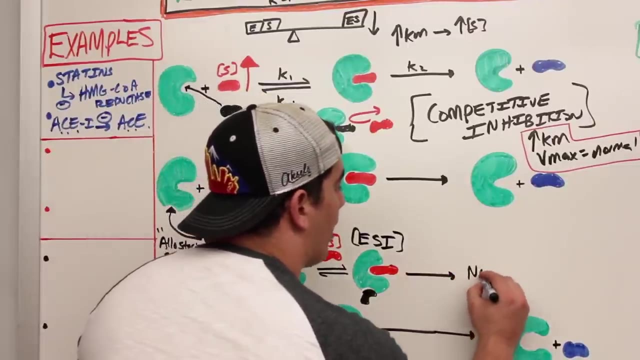 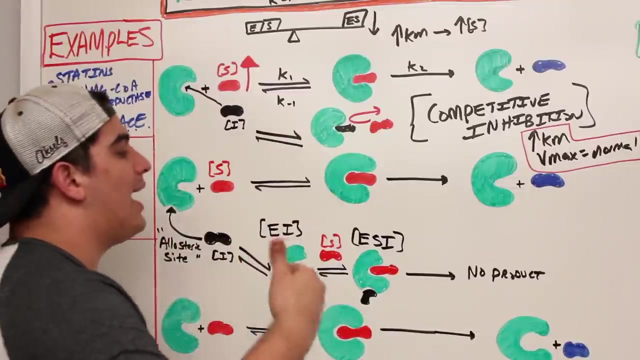 Here we have a enzyme substrate inhibitor complex. Holy crap, Can this guy ever get converted into this product? No, So this reaction will never produce product. So there will be no product formed from this reaction. But if by some possible way this inhibitor is released, 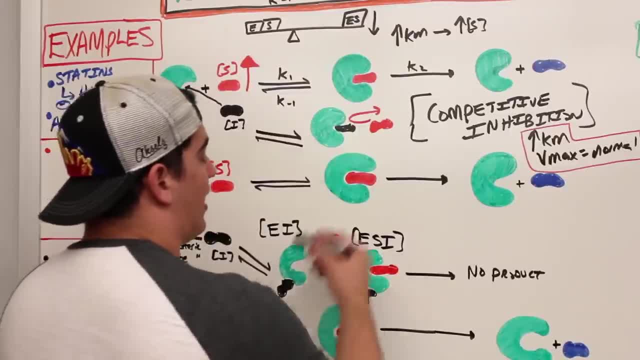 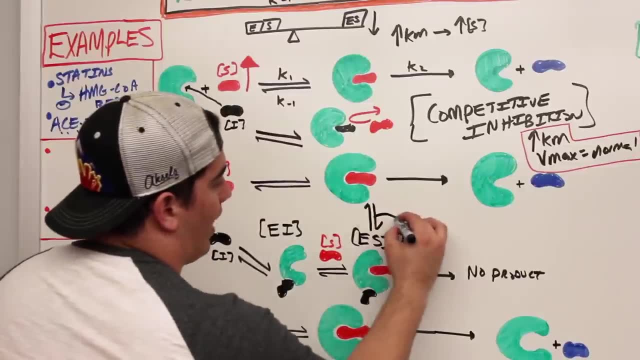 So let's say, I draw here an arrow coming up to the free- to this enzyme substrate, not free enzyme, enzyme substrate. So now, look, I have this reaction here and what did I- let's say I release out out of this. What did I release? 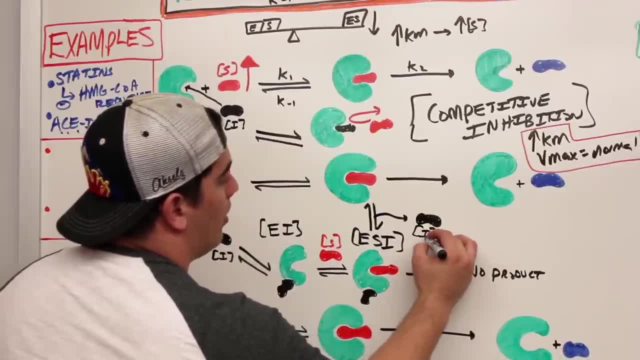 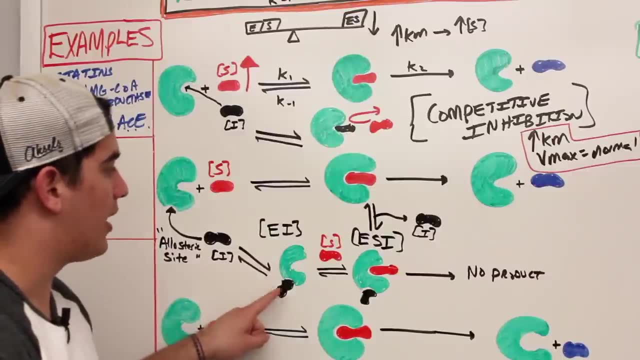 I release out this inhibitor, By some way, I get rid of the inhibitor. So the inhibitor is binding onto the allosteric site, forming the enzyme inhibitor complex. but the enzyme inhibitor can still bind with the substrate. Then, when it binds with the substrate, we have 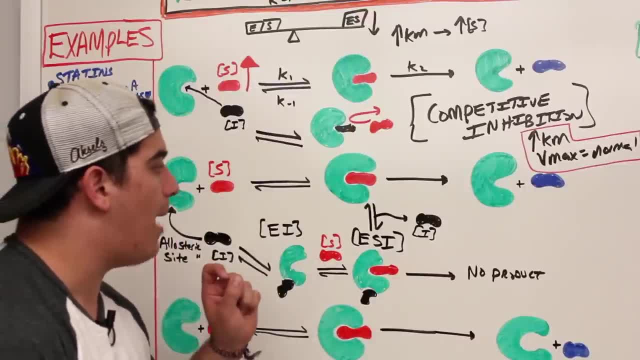 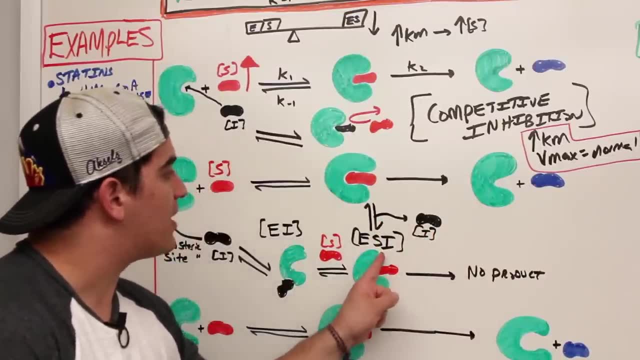 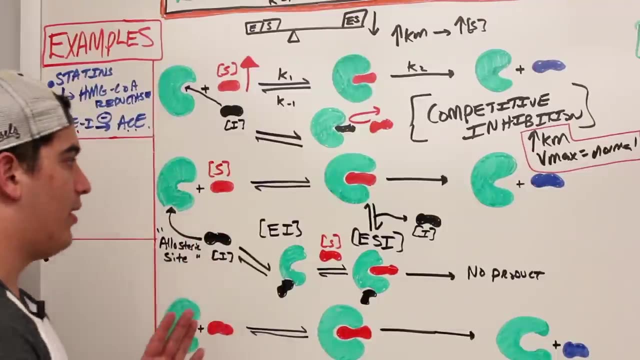 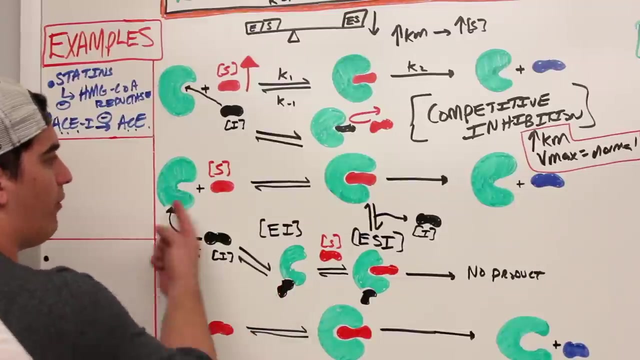 an enzyme substrate inhibitor complex. What can happen? then The inhibitor can be released. and if the inhibitor is being released, then what happens? I form my enzyme substrate and then the reaction can occur and then make more product. But look what's happening in this reaction, If you think about it: non-competitive inhibitors: they can bind on to the free enzyme. 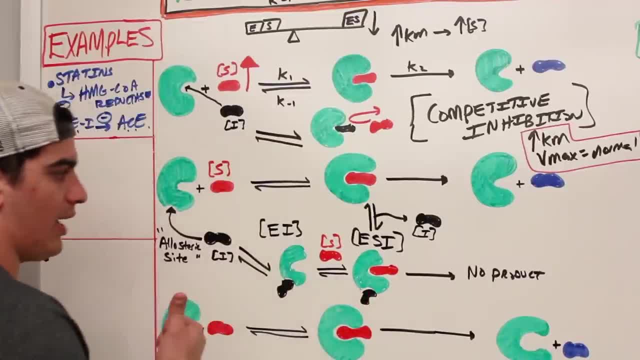 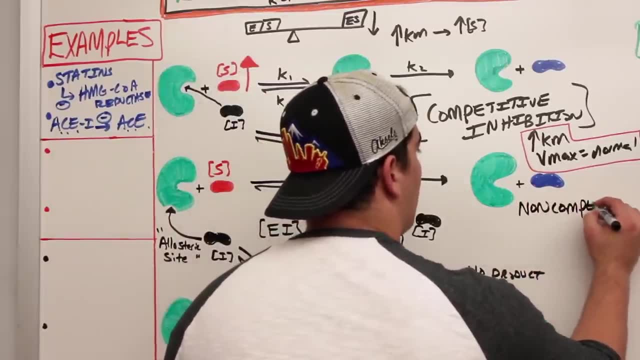 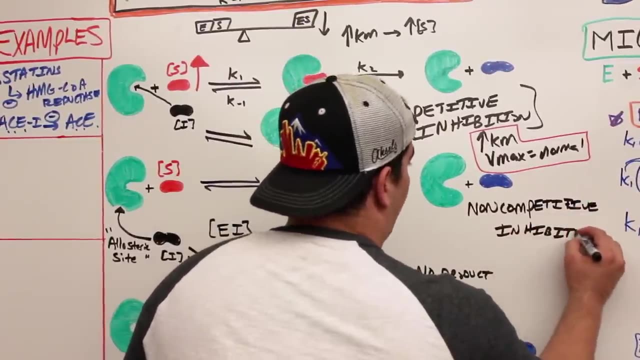 but they can also bind onto the enzyme substrate complex. So again, we're going to start with the free enzyme and then the enzyme substrate complex. what is this one right here? This is called non-competitive inhibition. Okay, now we have to look at something else here. So when we look at non-competitive 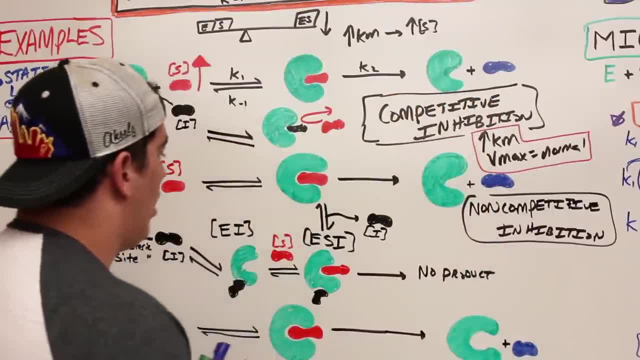 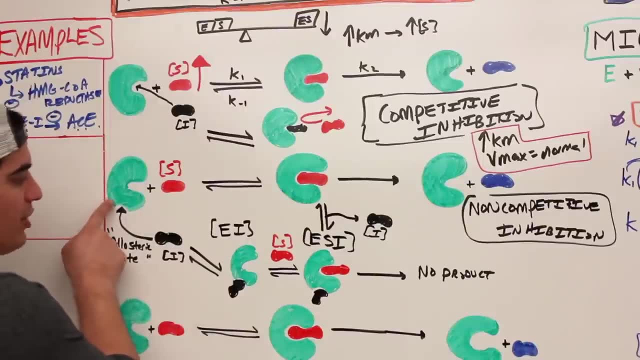 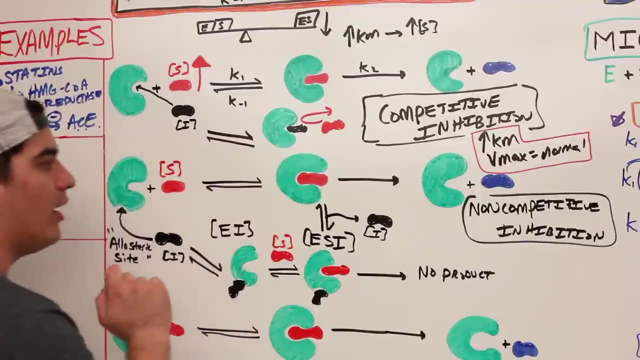 inhibition as compared to competitive inhibition, because we're still able to form enzyme substrate. so, in other words, because this reaction is proceeding in this way that it's still making enzymes. so this can go two ways. it can go this way or can come this way. technically, our equilibrium is not thrown off. We're. 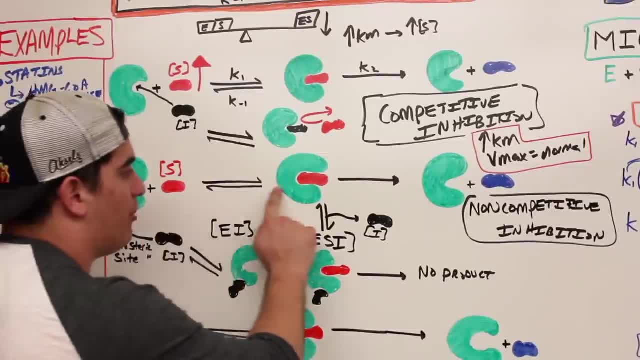 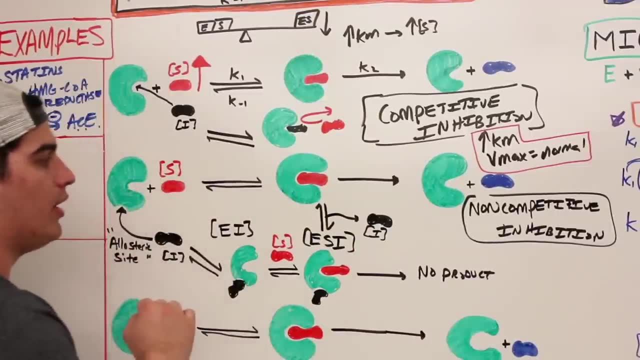 still in equilibrium with these reactions. So because this reaction can proceed this way and it can come all the way up through, this way, our equilibrium isn't thrown off. So because the equilibrium isn't thrown off, we did not change the Km. So the Km for this reaction is not thrown off. So the Km for this. 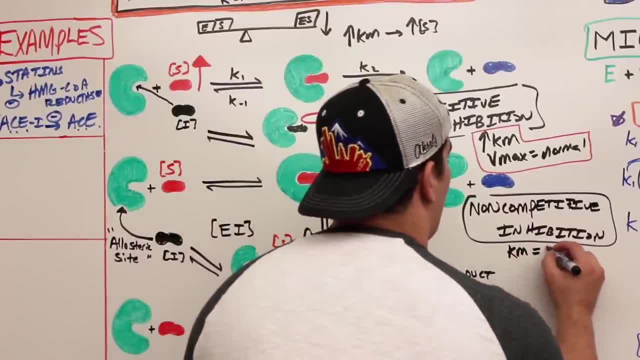 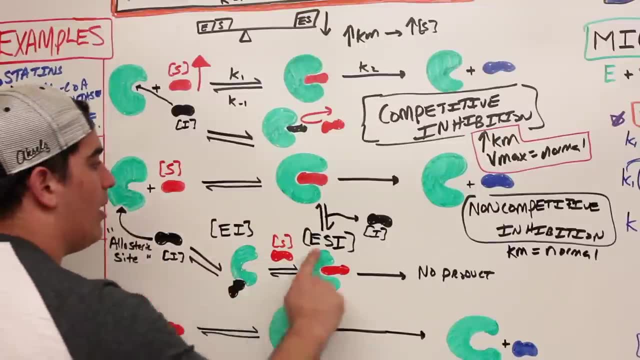 reaction remains unchanged. I'm going to put normal right or unchanged. So because? again one more time: why is the Km normal? Because the equilibrium for this reaction is not changed, It's not shifting from one side to the other, It's. 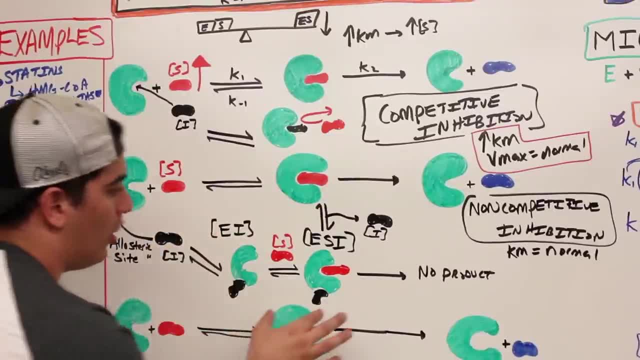 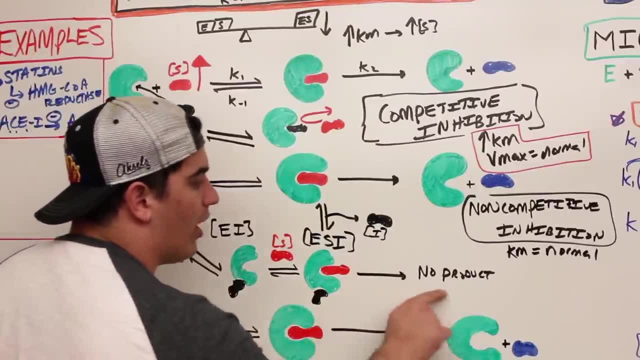 favoring a normal equilibrium. However, look what happens here. Because this inhibitor is binding on to that enzyme with the substrate. can you form product all the time? No, Some product isn't going to be formed. and then look what happens. 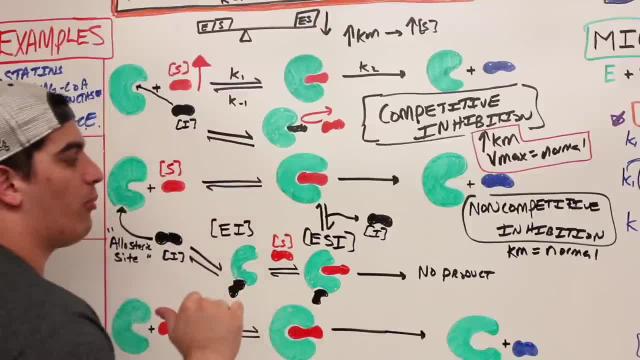 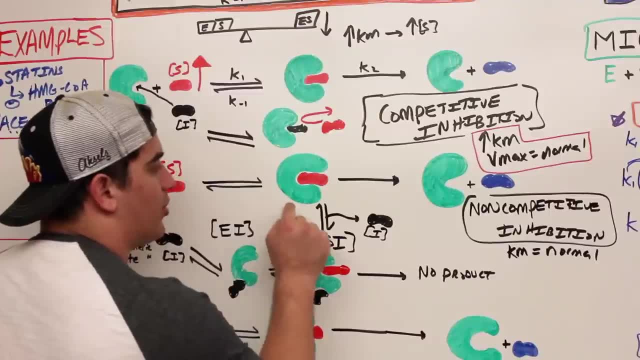 Some of it you can make enzyme substrate and some of them you can actually form product. But at some point in time, not all of this enzyme will be in the form of enzyme substrate complex. So in other words, you'll never be able to have all of your enzymes bound to substrate. 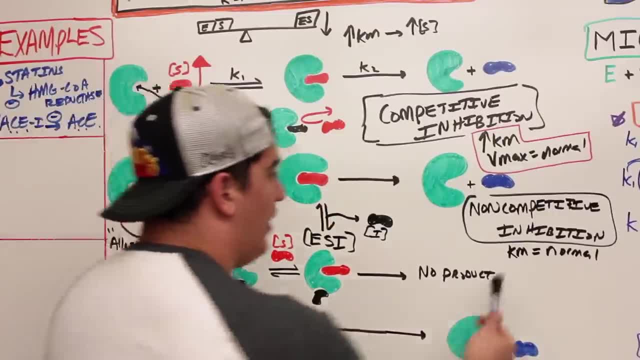 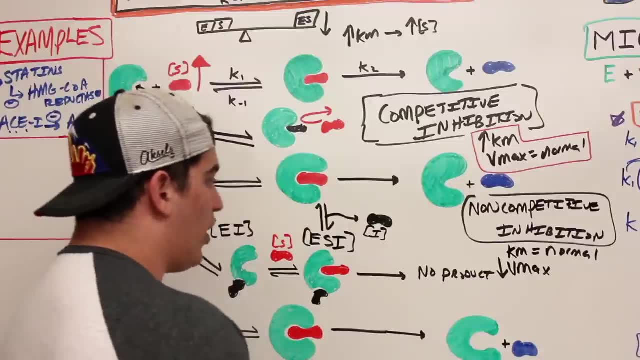 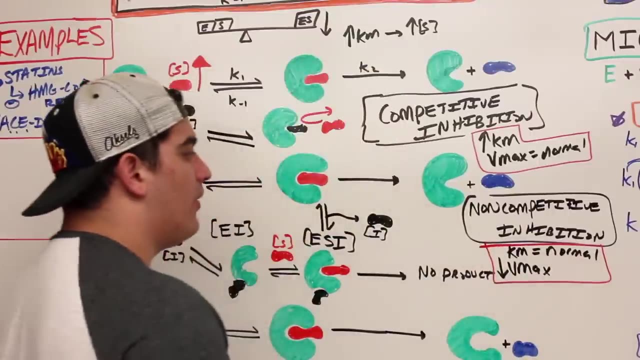 So what does that mean? I'll never reach Vmax. So Vmax decreases in this point. So Vmax decreases. So these are really important concepts. Let me highlight these guys again. These are really really important things again. So what happens in non-competitive inhibition? 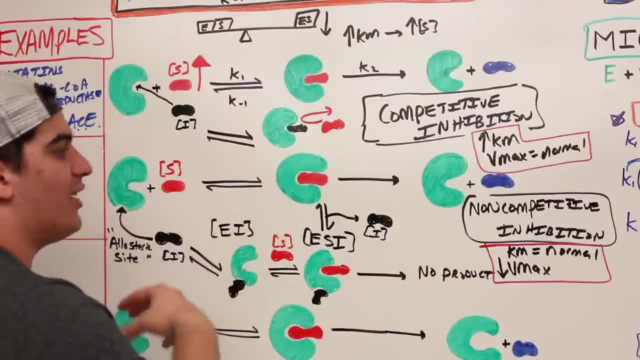 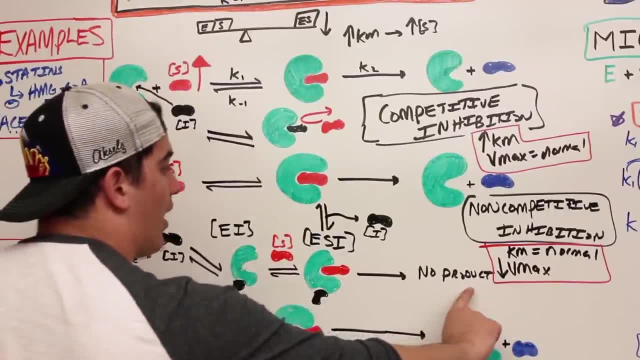 Km is normal. Why? Because the normal equilibrium of this reaction is not changed or it's not favoring one side or the other. Vmax decreases. Why? Because some of this reaction will form no product and you'll never have the enzyme. 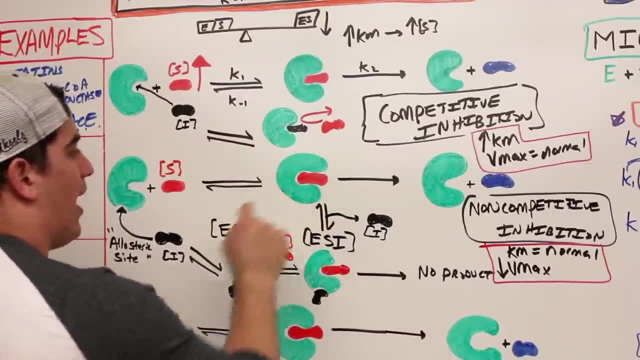 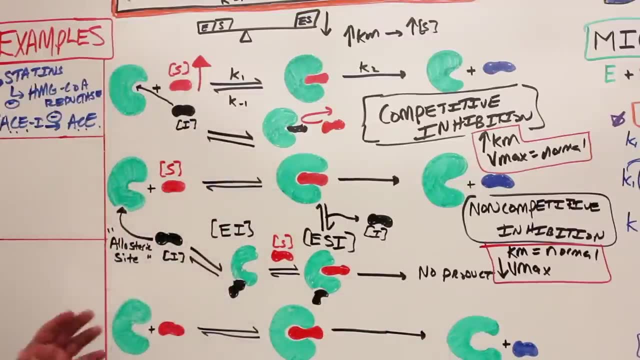 All of our enzymes. never, never will all the enzymes be bound to substrate or to be completely saturated, So it never reaches Vmax. All right, Now that we've done that, let's give some practical applications of certain types of non-competitive inhibitors, like physiologically. 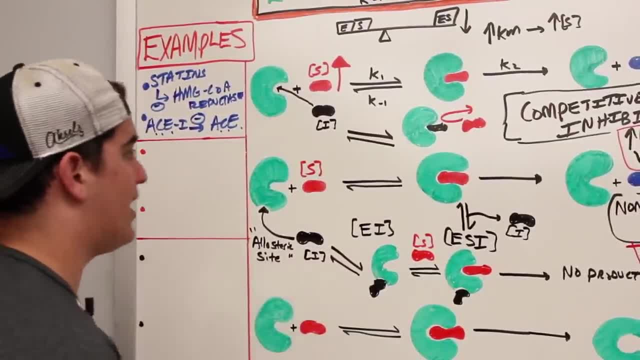 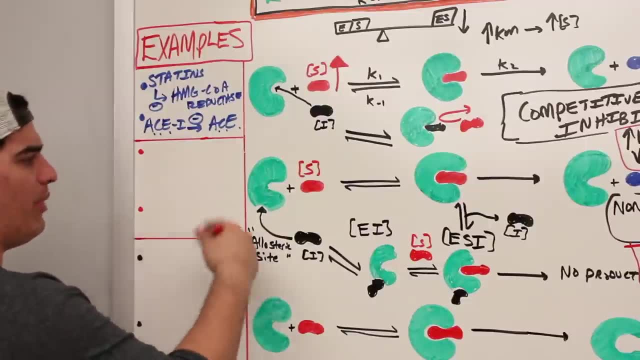 So one of them is actually used a lot in certain cases, maybe certain types of depressions or certain things with catecholamines, norepinephrine, epinephrine, and these can be called monoamine oxidase inhibitors. 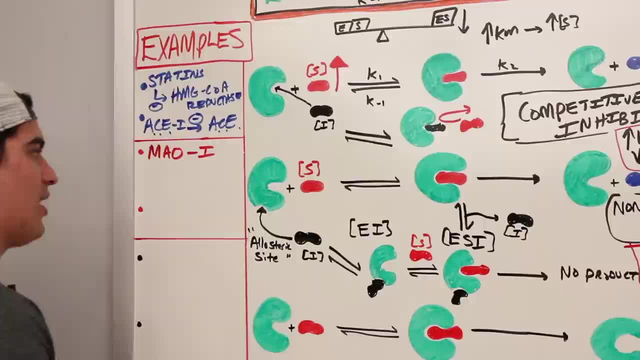 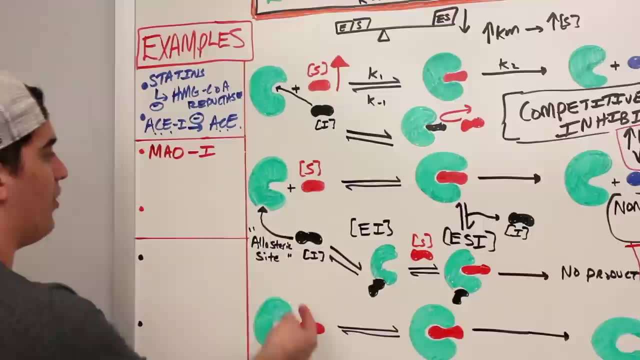 So monoamine oxidase inhibitors. There's many, many different types of monoamine oxidase inhibitors. We're not going to go into each one, but basically, what can they do? They can bind on to certain allosteric sites of monoamine oxidases. 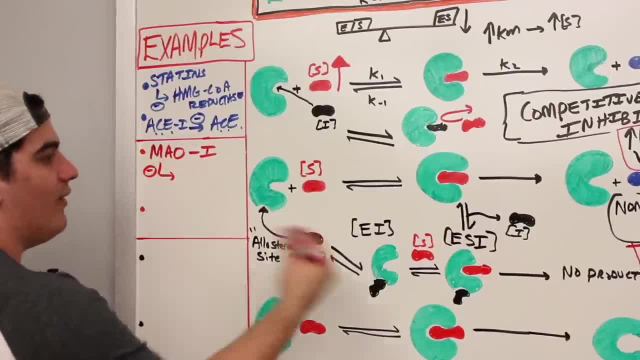 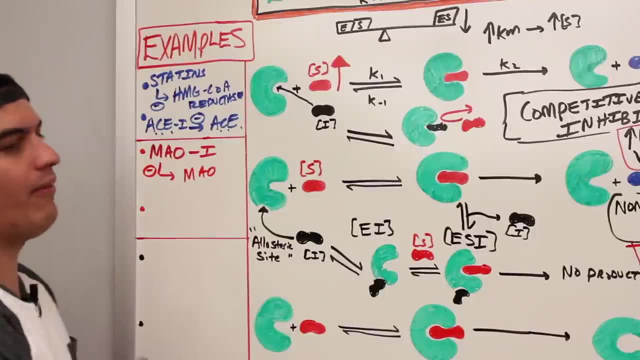 And what do they do? They inhibit the normal activity of that enzyme, right? So it inhibits the monoamine oxidases which are important for being able to break down norepinephrine, epinephrine, dopamine, so on and so forth. 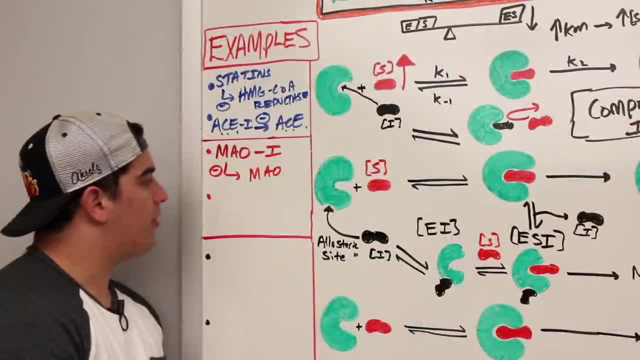 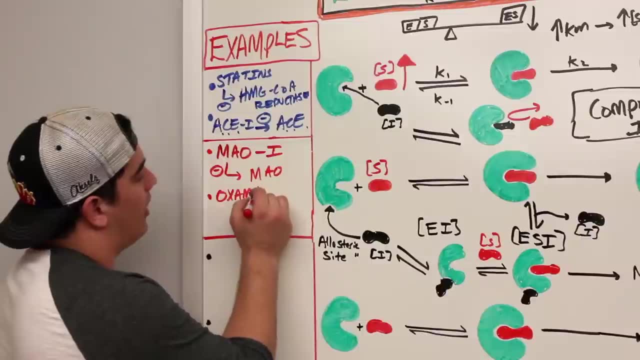 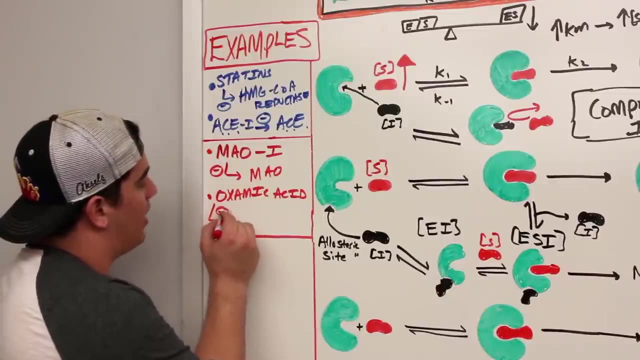 Okay, That's one example. Another one could be what's called Oxamate, Oxamate or oxamic acid. So I'm going to put oxamic acid, And what this enzyme does is it inhibits a specific enzyme which is called lactate dehydrogenase. 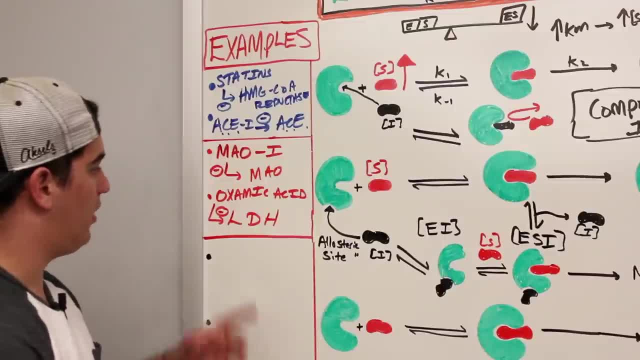 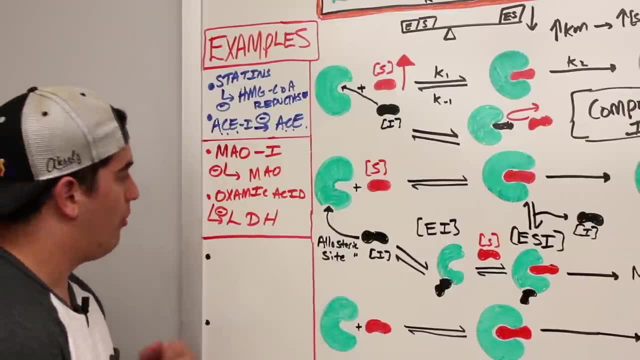 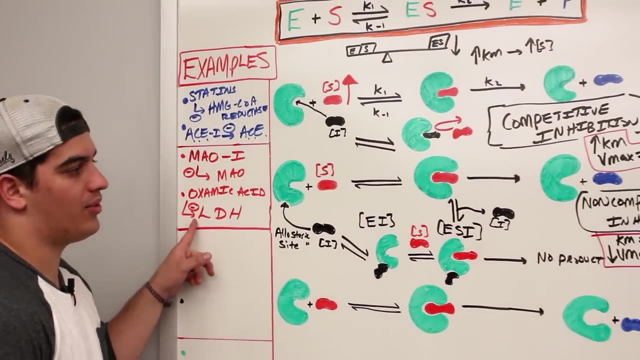 So oxamic acid or oxamate can basically inhibit this enzyme called lactate dehydrogenase. How, Binding on to the allosteric site and affecting the normal production of product. How is that going to affect us physiologically? Lactate dehydrogenase is actually important for being able to convert lactate into pyruvate. 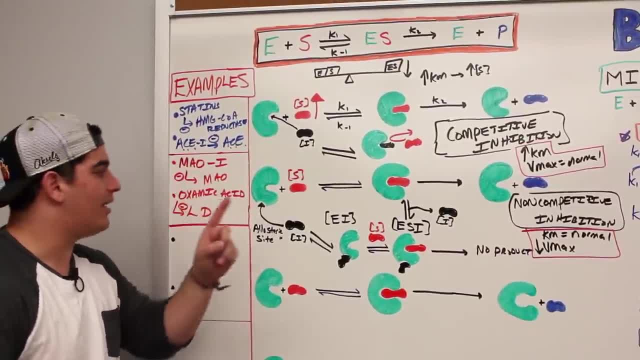 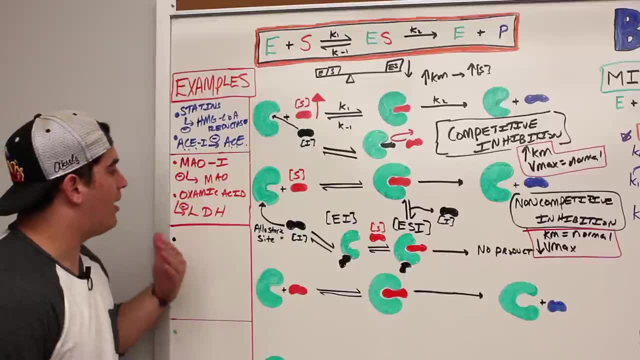 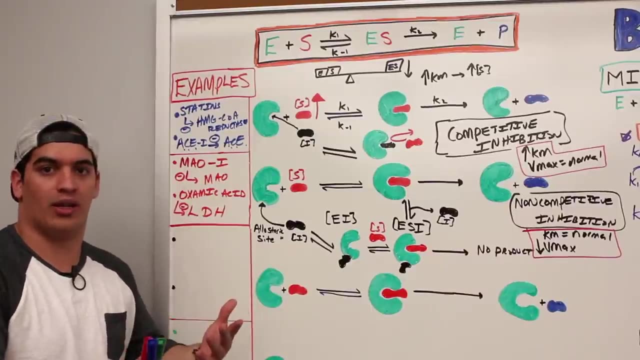 And pyruvate can actually get converted into glucose And if lactate is going into forming glucose, that's called gluconeogenesis. So oxamic acid is a normal, non-competitive inhibitor of lactate dehydrogenase or an overall pathway called gluconeogenesis, which is needed to be able to put glucose into our bloodstream. 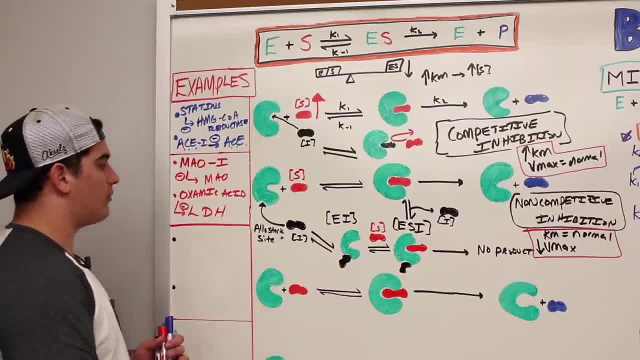 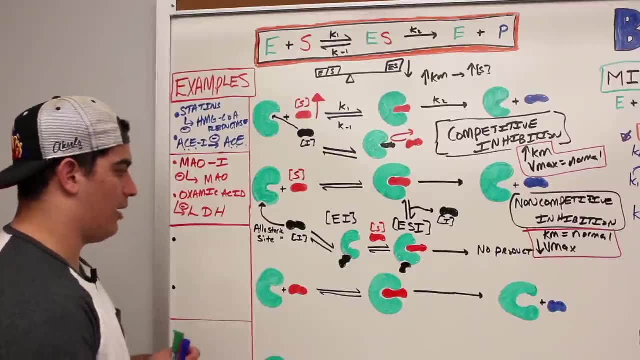 All right. So that can affect our glucose levels, All right. So that's an example there. Let's do the next one here, And this is going to be called uncompetitive inhibition. So uncompetitive inhibition is kind of like non-competitive, but here's where the difference is. 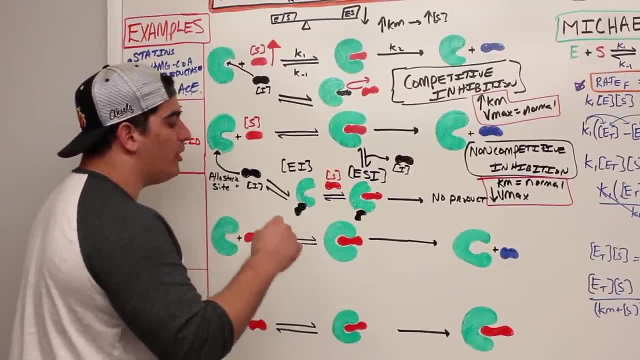 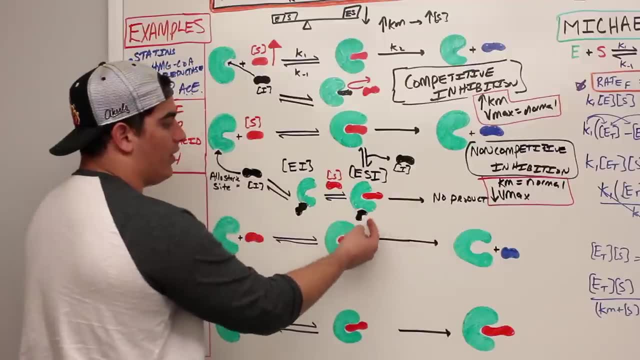 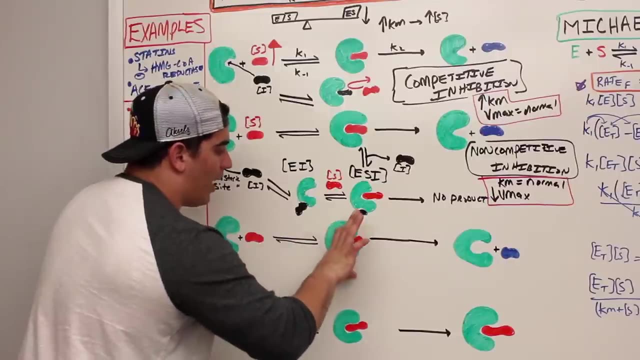 The uncompetitive inhibitor only binds on to the enzyme substrate complex, whereas the non-competitive the inhibitor could bind on to the enzyme substrate complex or the free enzyme In uncompetitive. when the enzyme binds to the substrate, then they make an allosteric site. 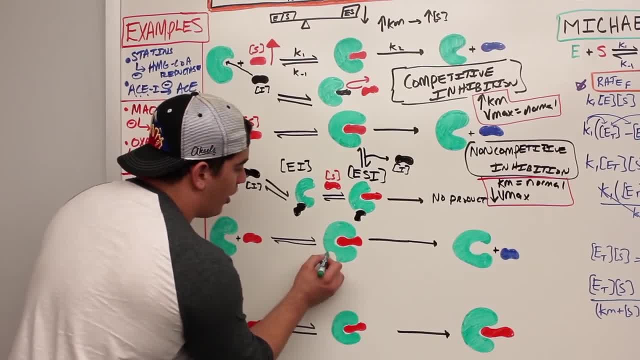 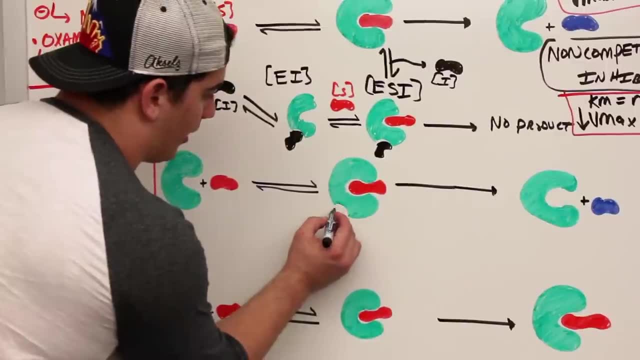 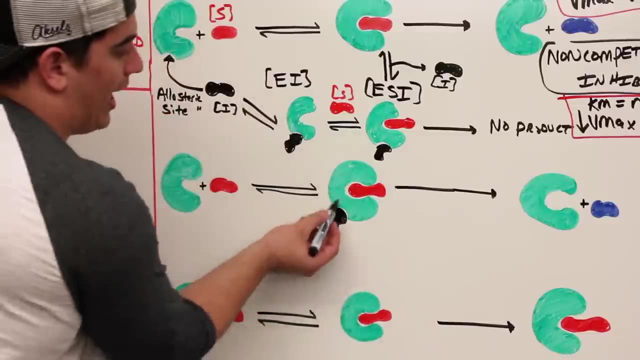 Okay. So there's an allosteric site that's only opened up whenever the enzyme is bound to the substrate. And then look who comes in and plugs in here. Now we have our uncompetitive inhibitor. If the uncompetitive inhibitor binds on to this, what do you get then? 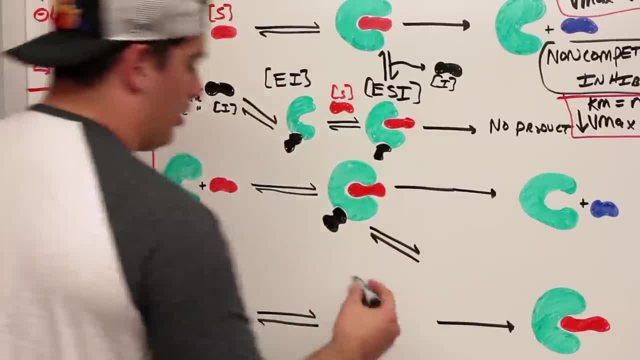 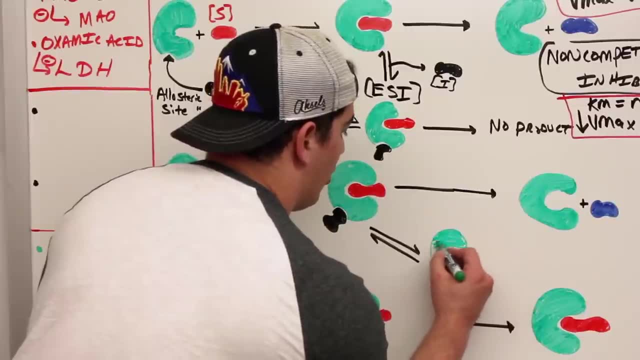 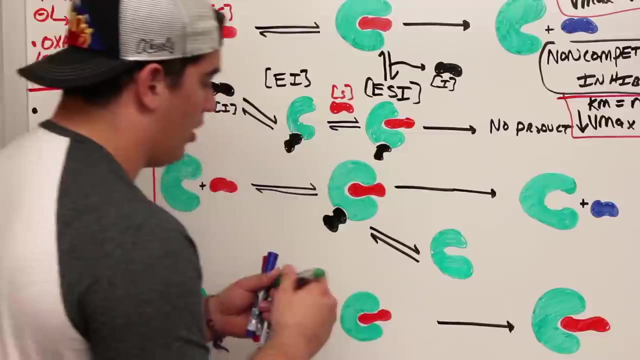 We'll get A Look at this, Look at this new enzyme over here. We'll get a new enzyme over here And this is going to be bound to the substrate, right, which is going to be bound in the active site. And then, when it's bound into the active site again, what happens? then it changes its shape to form a little allosteric pocket there. 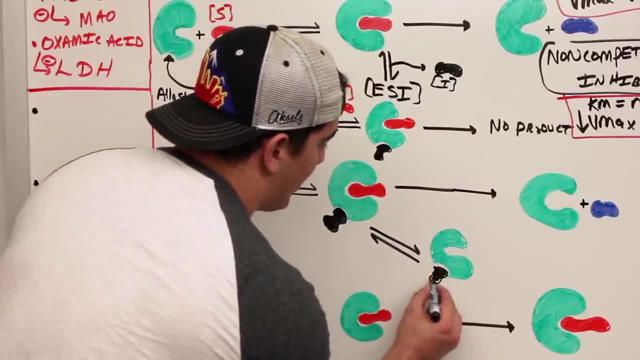 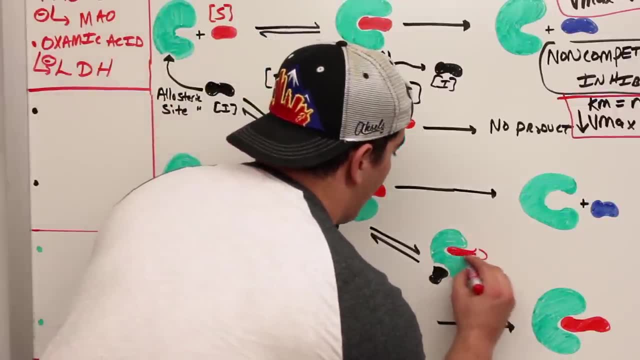 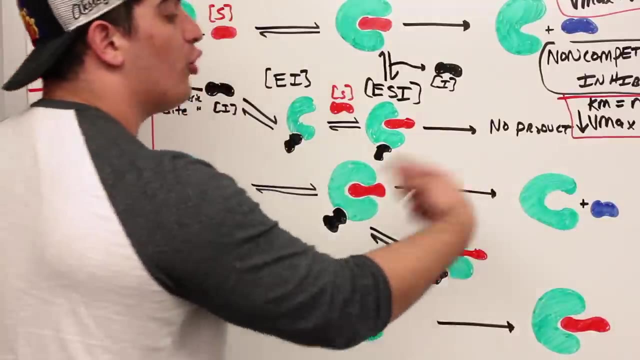 And then the uncompetitive inhibitor comes in and binds into that allosteric site, And then the substrate is still bound into this active site here. Now where's the problem with this? This enzyme is going to have a hard time turning the turnover rate, in other words, 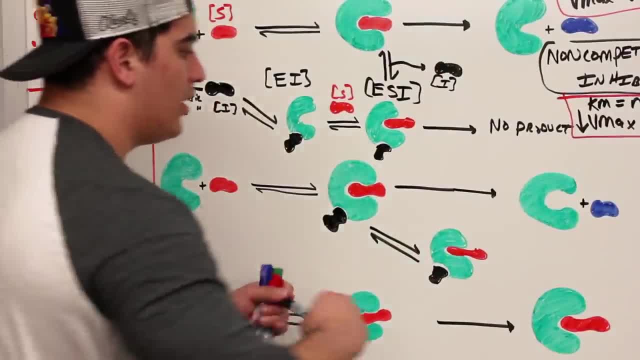 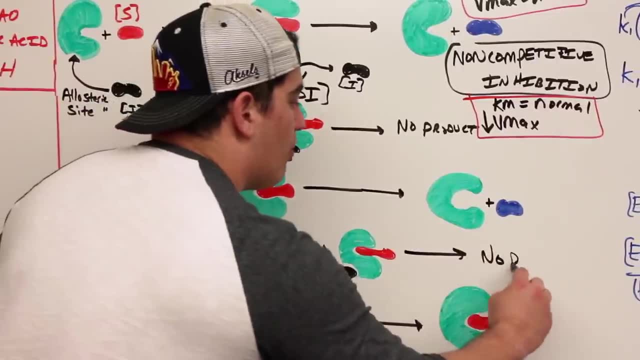 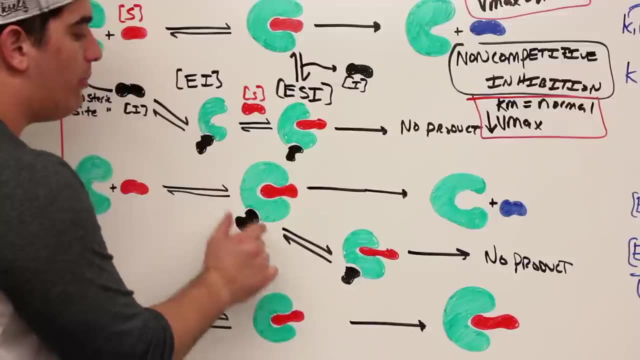 So, in other words, the product formation is going to decrease. So me being able to form product from this reaction is not going to happen. Same thing like this one. What do you get? No product, Okay. So with this one it only. the inhibitor only binds on to the enzyme substrate complex. 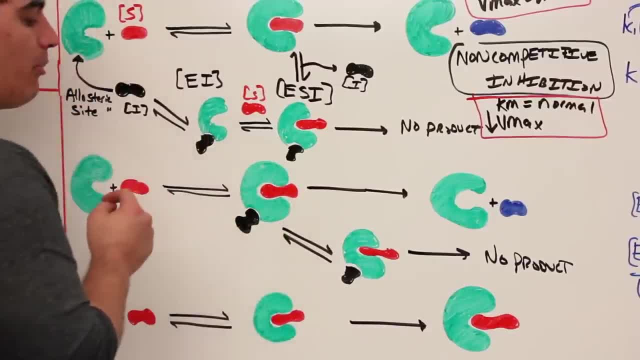 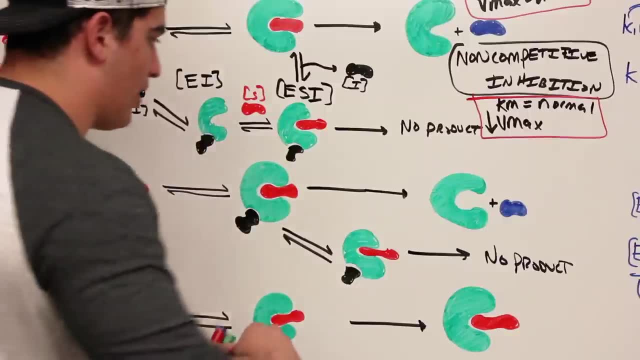 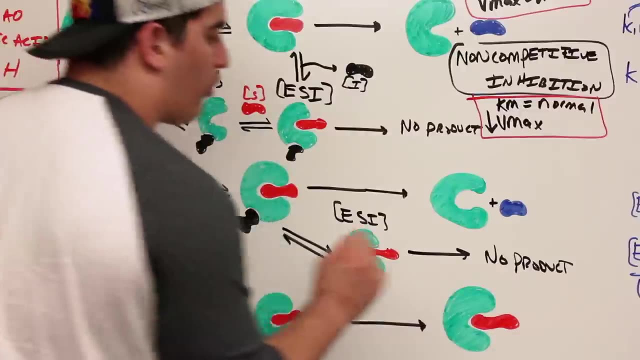 Why? Because when the enzyme is bound to the substrate, it opens up an allosteric pocket for the uncompetitive inhibitor to come in and bind And then you form this enzyme substrate inhibitor complex. So again, what is this guy here? Enzyme substrate inhibitor complex there, which will form no product. 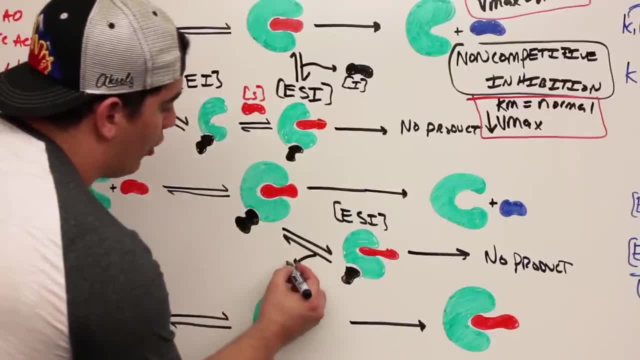 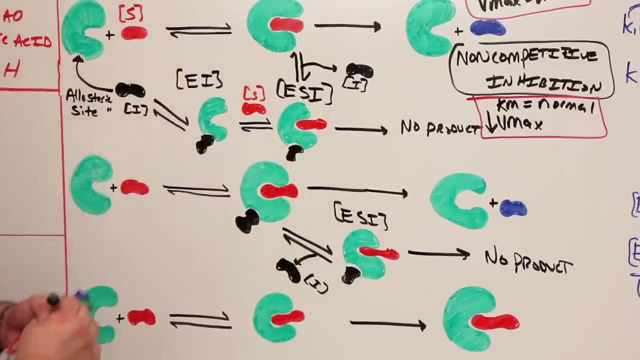 But if by some way you're able to release that inhibitor from the allosteric site, So let's say, here's your inhibitor And you're able to release that inhibitor from the allosteric site, You can form. let me actually get this guy out of here. 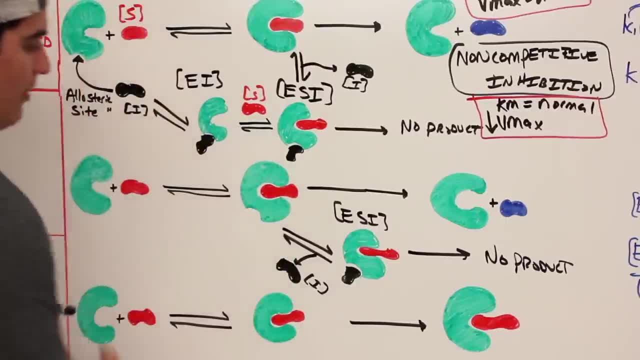 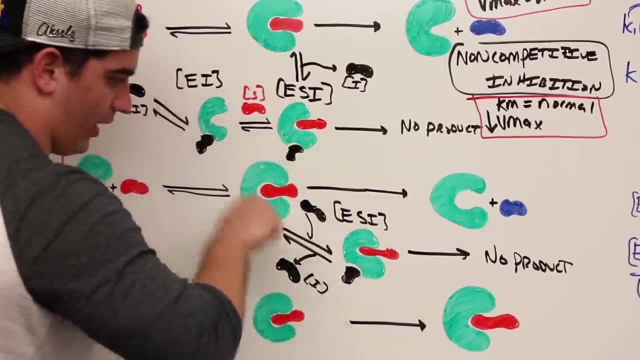 So now we have this free enzyme here, So we can actually have this guy coming in this way, So we can have the inhibitor coming in into this reaction. So going this way, Or we can have the inhibitor release coming to forming our enzyme substrate. 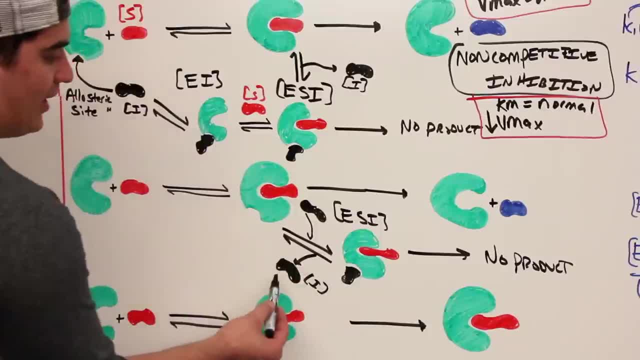 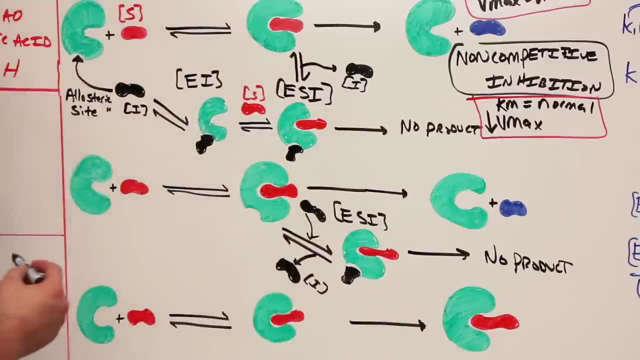 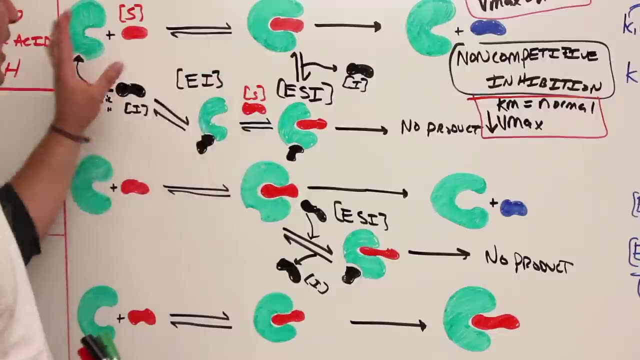 So if the inhibitor is released, then what do you get? You get your enzyme substrate which can progress to forming product. Now, with the noncompetitive, we said that the normal Km, like the equilibrium of going from enzyme substrate to enzyme substrate complex, wasn't affected. 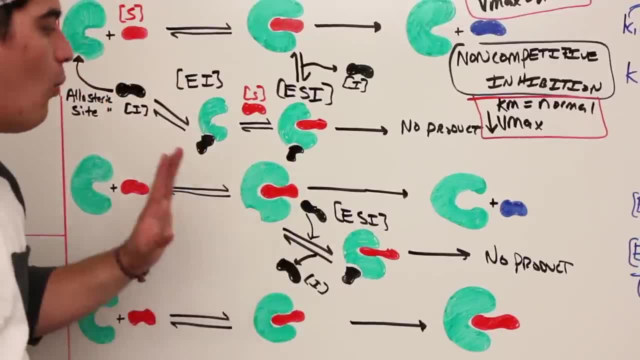 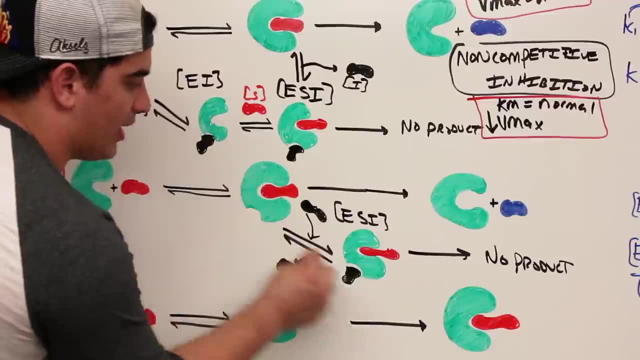 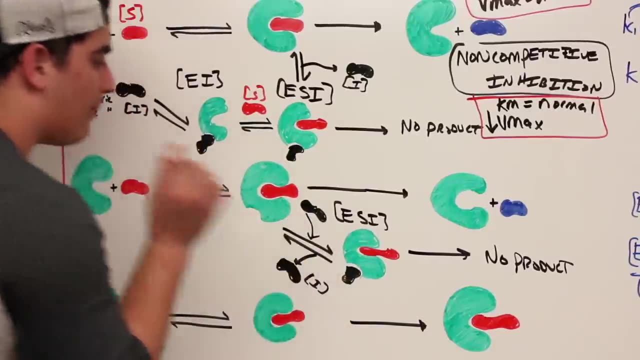 However, in this reaction, it is Why, If you think about it, if the inhibitor is binding onto the allosteric site on the enzyme substrate complex and making enzyme substrate inhibitor, what's happening to the normal concentration of our enzyme substrate, Our normal enzyme substrate? 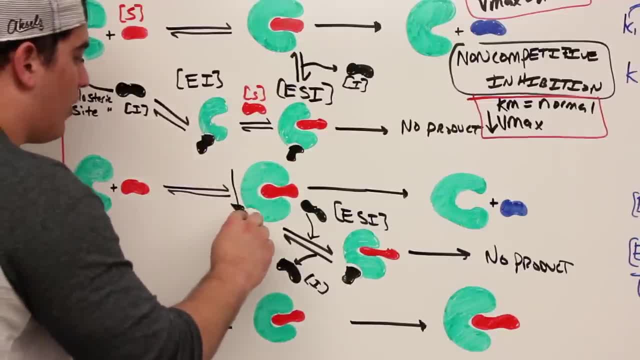 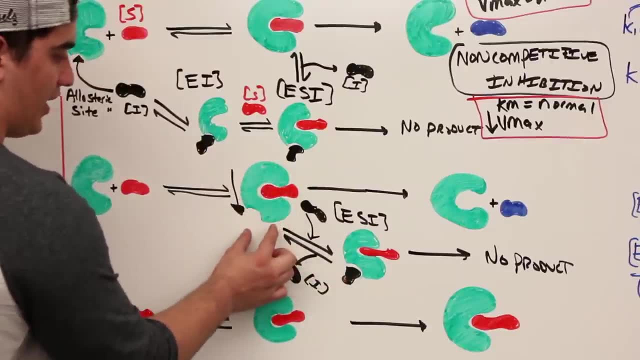 It's decreasing. So if the normal concentration of our enzyme substrate not bound to the inhibitor, not this one- if this amount is decreasing- right, because a lot of this is bound in this form, then what does Le Chatelier's Principle say? 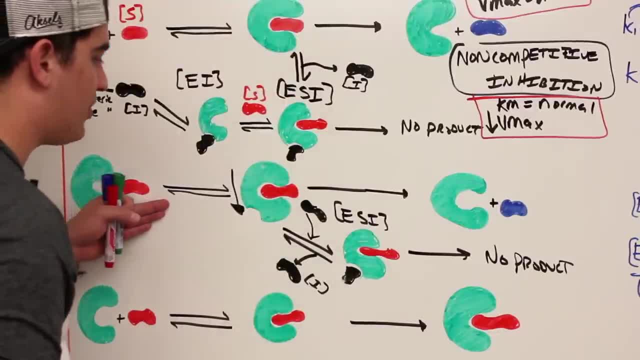 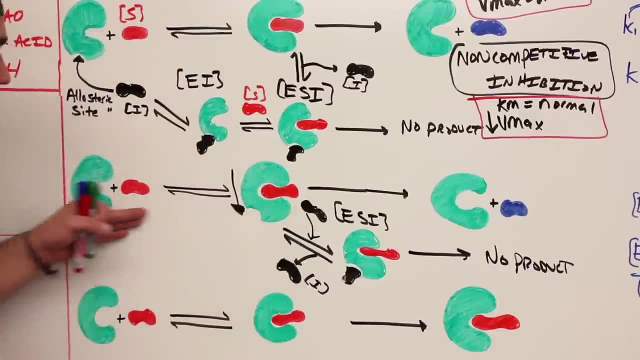 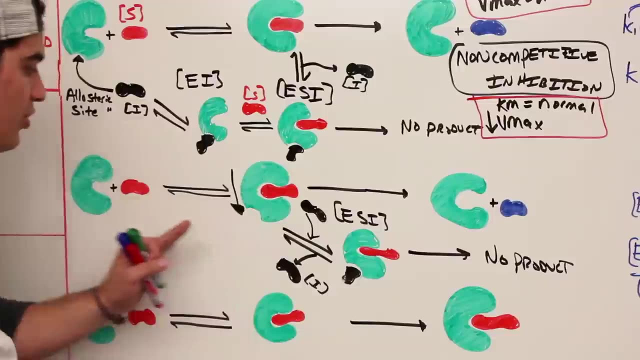 It kind of goes back to this: The reaction is going to proceed to the right. So now, when the reaction starts proceeding to the right, what starts happening to the concentration of my enzyme substrate? Well, the substrate concentration starts going down. And as the substrate concentration starts going down, as you're working this way, 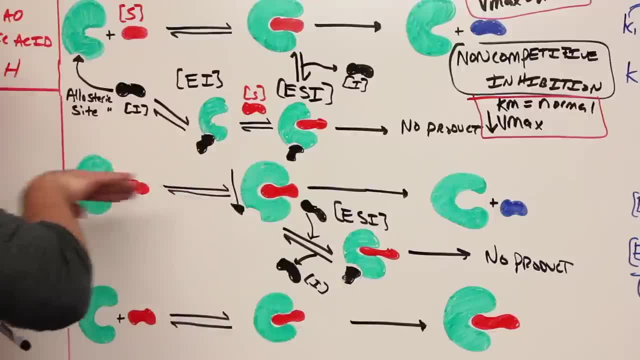 so again, what's happening to the substrate concentration, as this reaction is progressing this way. So I'm going to draw it with red here, As this reaction is progressing this way, according to Le Chatelier's Principle, because again what's happening. 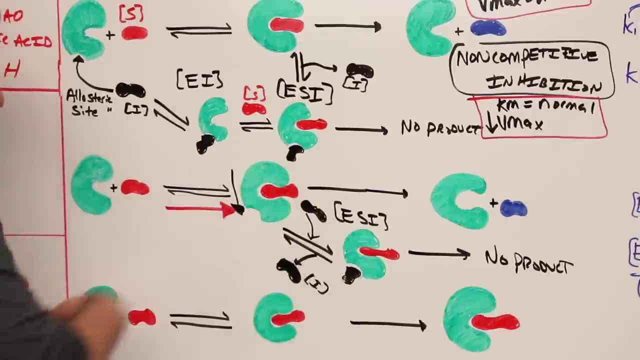 The normal enzyme substrate concentration is decreasing, The reaction is going to shift to the right. So what happens to the substrate concentration? It starts decreasing. So as the substrate concentration starts decreasing, what starts happening to the Km? Well, it goes back to that concept. 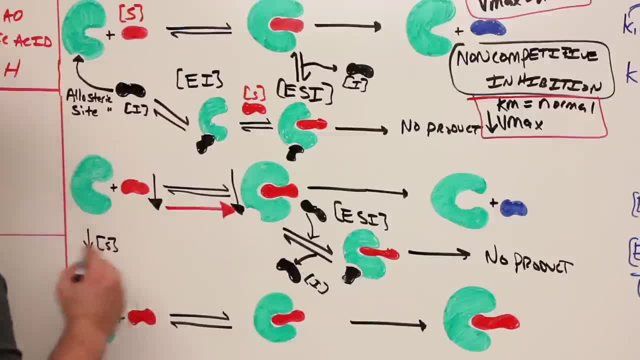 Whenever there is low substrate concentration, we said in the Michaelis-Menten equation video that it does what to the Km? It decreases the Km right. So now, because the substrate is moving to form enzyme substrate. what's happening to the Km of this enzyme? 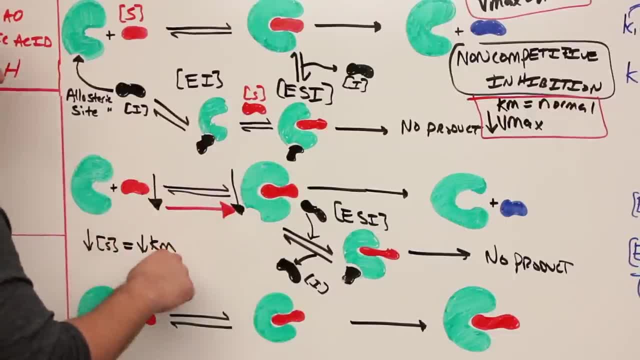 It's decreasing. Well, decreasing Km means what It means: it will accommodate less substrate. So whenever this event changes, because the substrate concentration is going down as the reaction is proceeding to the right, the substrate concentration goes down and now the Km goes down because the enzyme is dealing with less substrate. 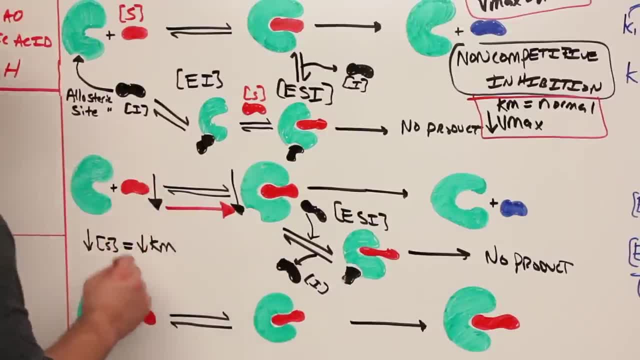 Okay, So this is again a measure of infinity. So now, what will happen to the affinity? again, If the Km is going down, it's going to have more affinity for the remaining substrate, Alright. So what happens in this reaction? And this one is uncompetitive. 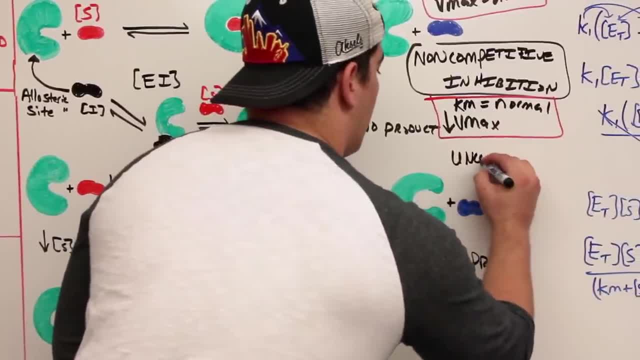 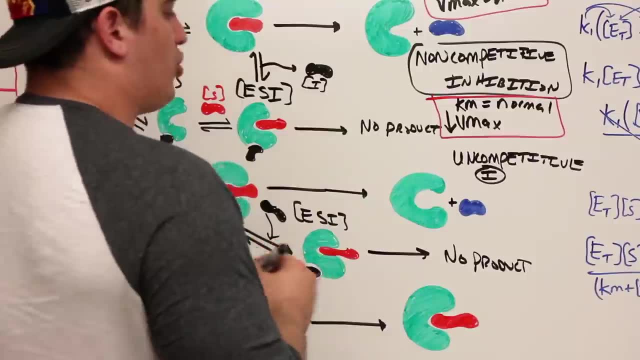 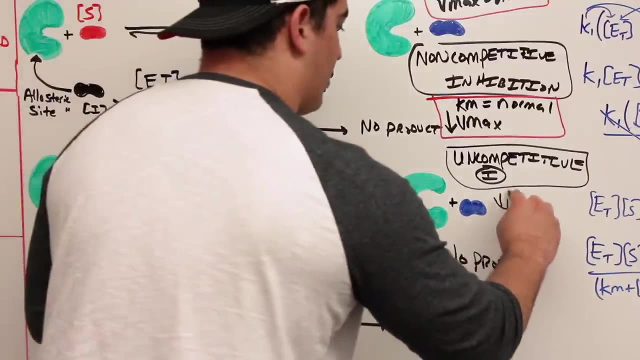 Let's write this one down. This one is uncompetitive And I'm just going to put inhibition here. So what is uncompetitive inhibition happening here? So if we look what happened to the Km, The Km decreased. Okay, That's looking good. 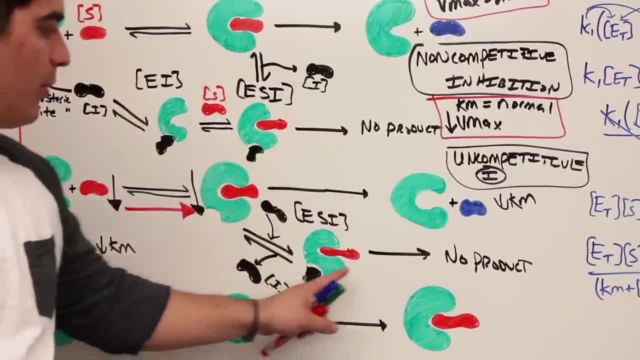 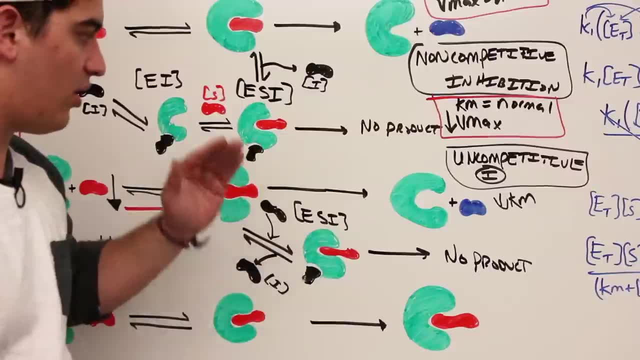 Then what? Remember? we said: when we form no product, what else are we forming here? No product. So that means that the normal amount of enzyme and product that we're going to form, our turnover, is going to start decreasing, right, So we're not going to make the full amount of enzyme substrate complex. 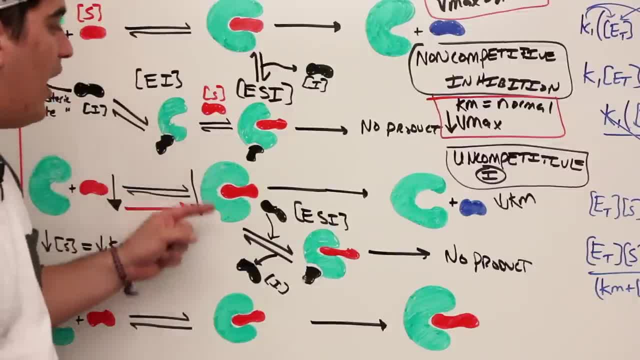 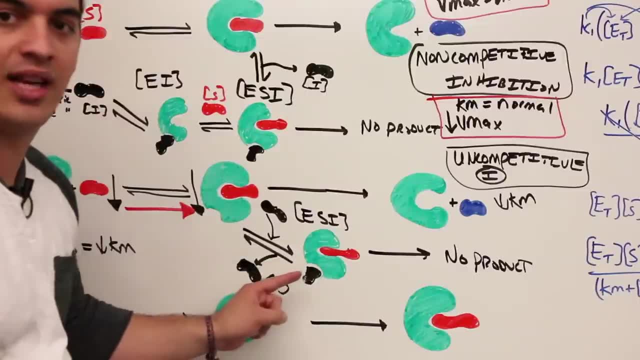 So, in other words, we will never have a point in the reaction in which the enzyme is completely saturated and bound with substrate. Why? Because some of it will always be bound to this enzyme substrate. Some of it will be in the enzyme substrate inhibitor form. 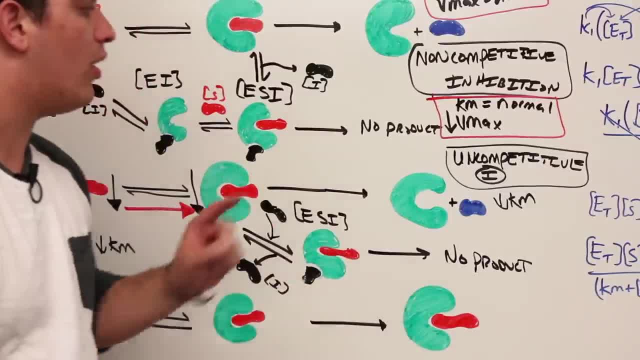 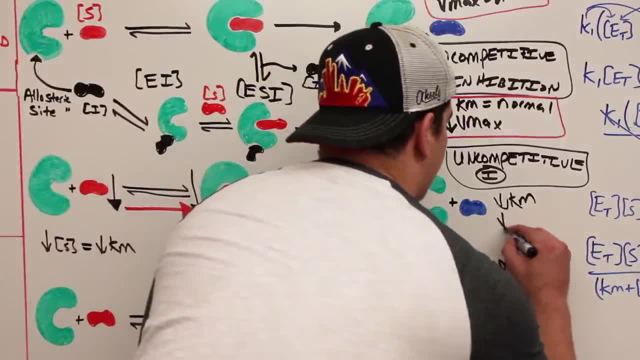 So if that's the case, then are we going to be able to make product with this reaction? No, So what happens to the Vmax? The same thing that happened with the noncompetitive: It decreases. So in this case, the Vmax decreases. 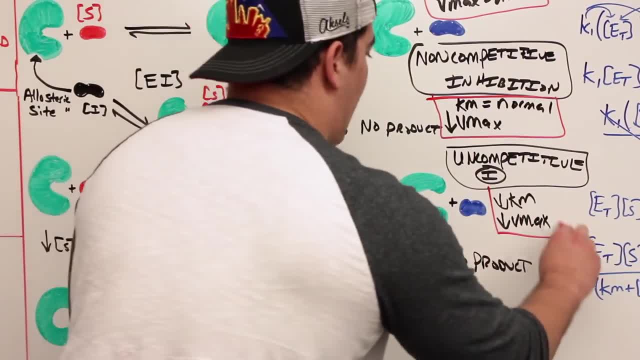 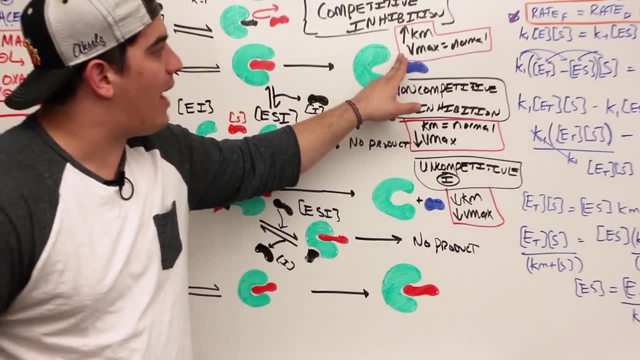 Okay, And again, this is another important concept here. So out of all these, let's quick recap, because we're going to do the last one here: Competitive is increasing the Km and then the Vmax is remaining the same. Noncompetitive inhibition: 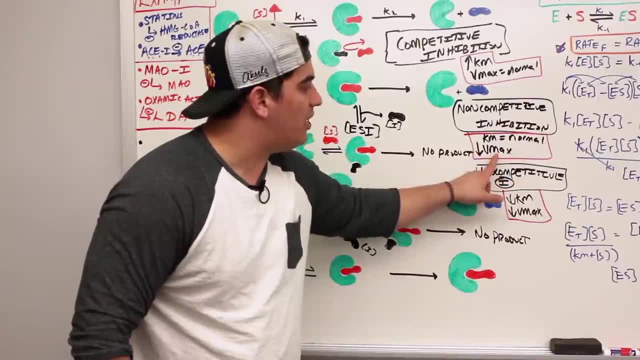 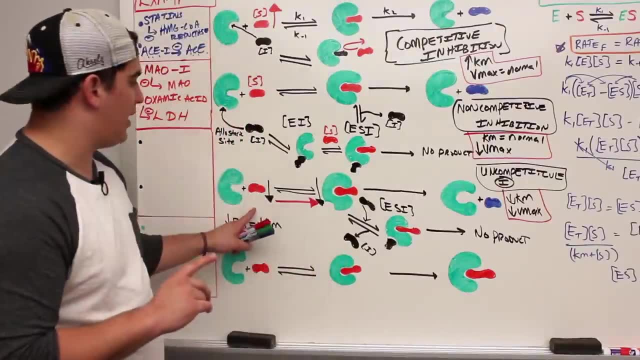 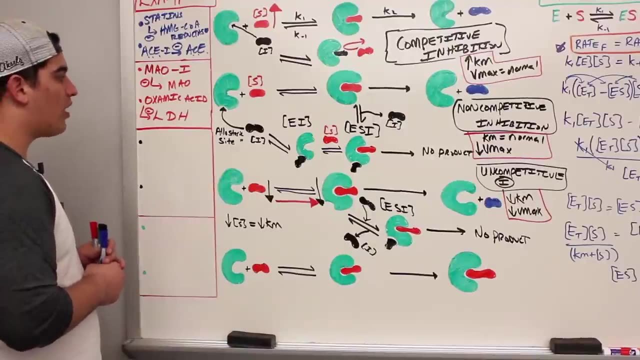 the Km is staying the same but the Vmax is decreasing. Uncompetitive inhibition: the Km and the Vmax are decreasing. Let me give you an example, real quick, of again two just uncompetitive inhibitors. So one of them is actually important within the glycolysis pathway. 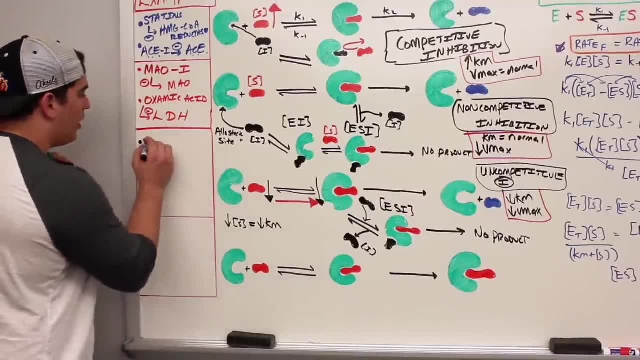 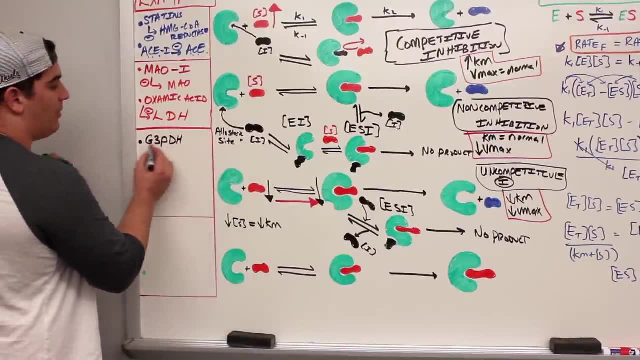 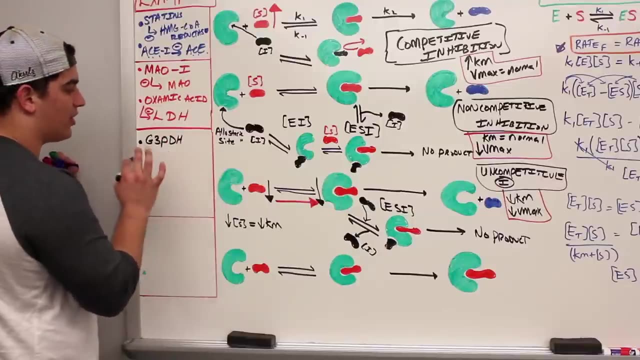 And this one is called glyceraldehyde 3-phosphate dehydrogenase, So this is the enzyme. This enzyme is normally important for being able to convert glyceraldehyde 3-phosphate into 1,3-biphosphoglycerate. 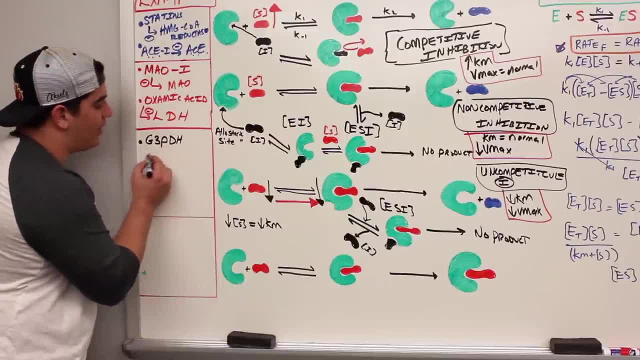 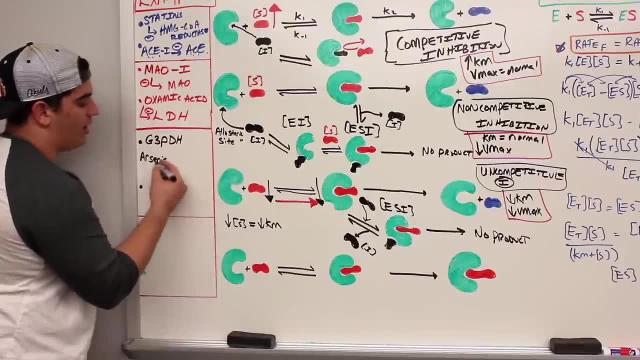 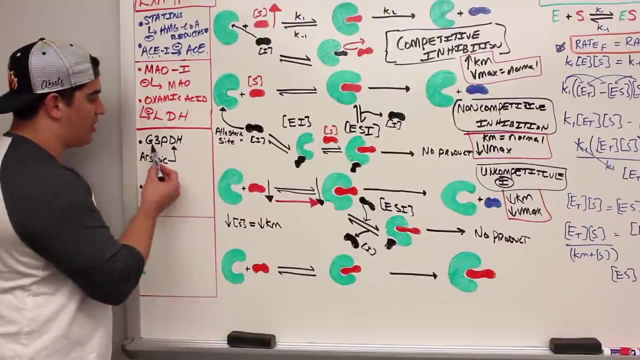 But what happens here is there's a certain type of like a poison. It's called arsenic or arsenate, So arsenic or arsenate, Basically what happens is that can actually bind on to the G3PDH, which is the glyceraldehyde 3-phosphate dehydrogenase. 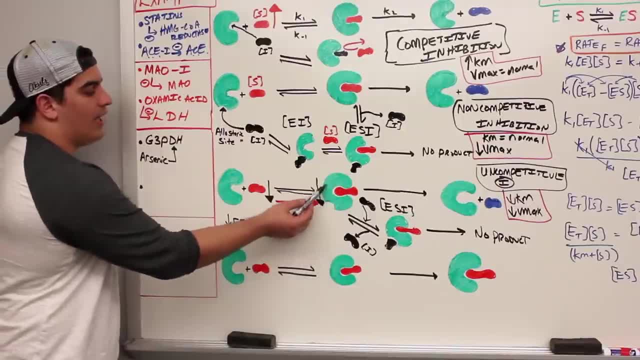 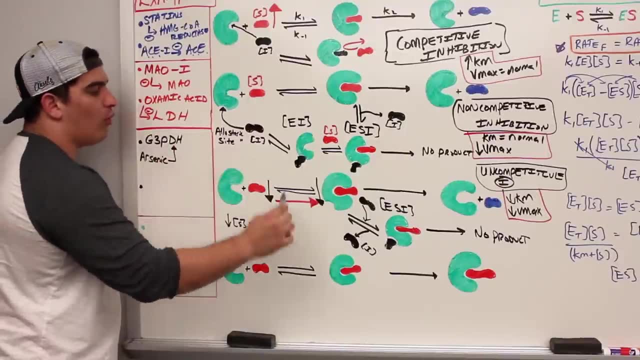 Where does it bind? It binds when the enzyme is bound to the substrate. What's the substrate? Glyceraldehyde 3-phosphate. But when arsenic binds, it affects the normal formation of the product. Okay, so that's one example. 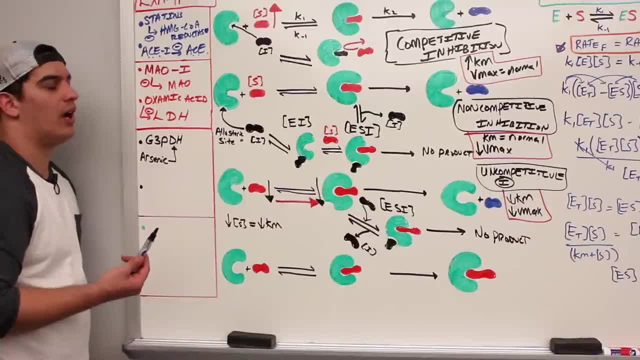 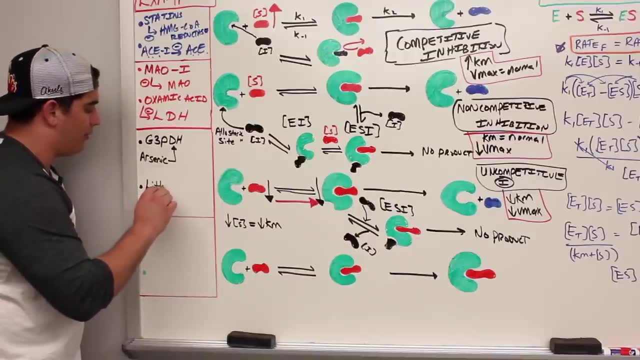 Another example of this one could be in bipolar disorder. They give people what's called lithium. So in bipolar disorder, so they give this an enzyme. They give it to individuals who have what's called bipolar disorder. They treat them with lithium. Why? 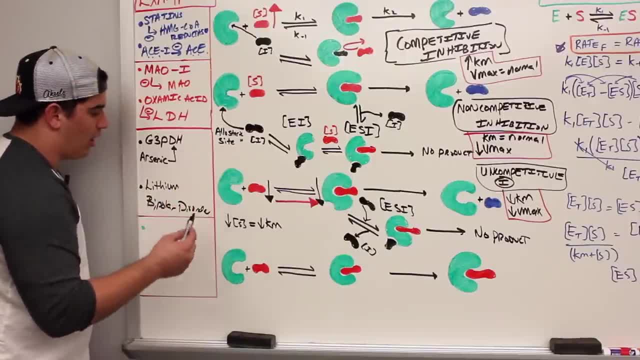 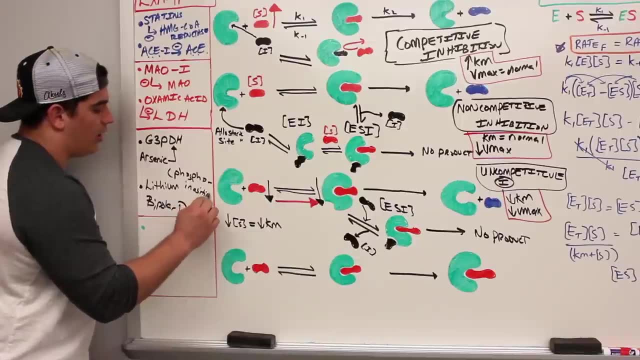 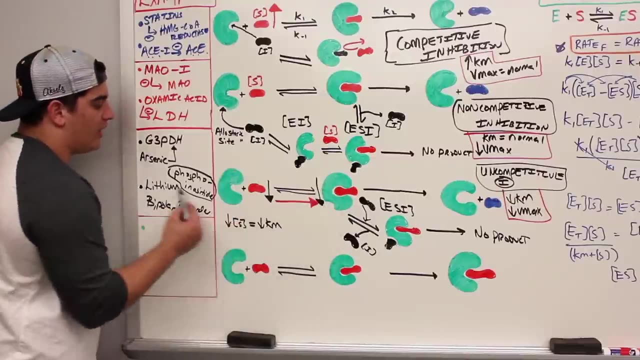 Because lithium binds on to a specific enzyme in this pathway, The pathway here. I'll write it out. It's called the phosphoinocytidide cycle or pathway. But basically what lithium does is it binds on to the specific enzymes within this phosphoinocytidide pathway. when it's bound to the allosteric site. 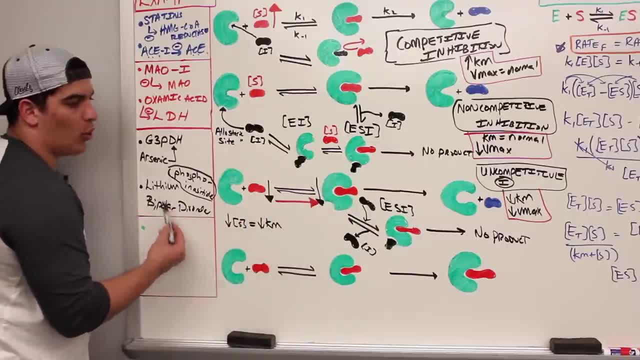 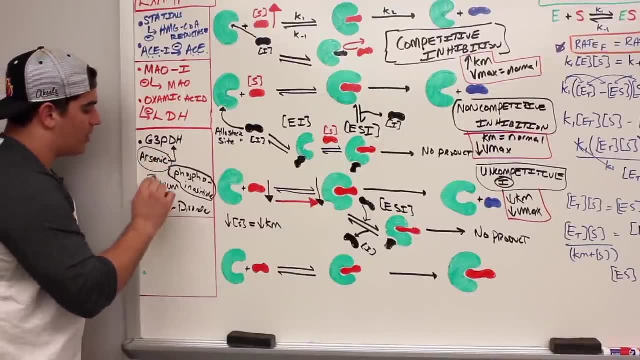 Right. So the enzyme is bound to that substrate And he affects the normal reaction and Km of that enzyme. So these are just again some examples. So again, what's a uncompetitive- Arsenic And what's another uncompetitive is lithium. 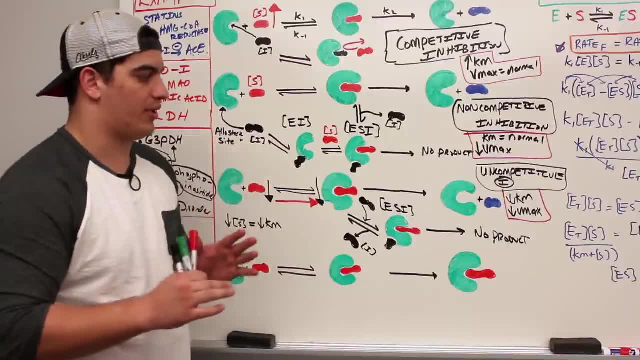 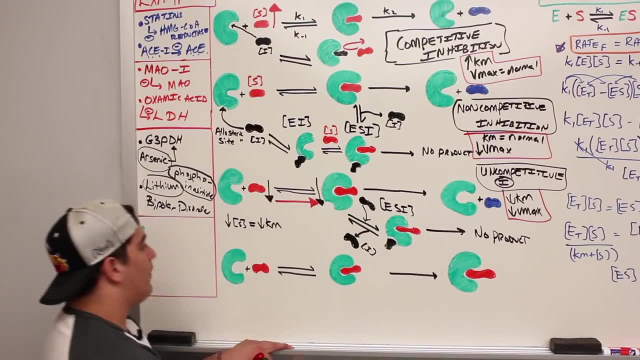 Competitive, noncompetitive, uncompetitive are all examples of reversible inhibitors. This last one we're going to talk about is an irreversible inhibitor. So how does this happen? All right, So if we look here, we have an enzyme And the enzyme is going to, it's going to want to bind on to this substrate. 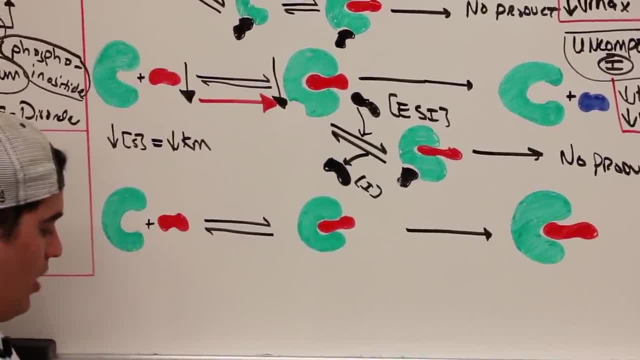 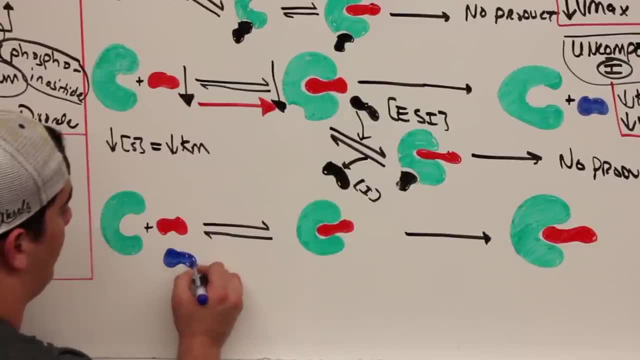 But let's say here, in this case, I put a inhibitor here, So here's this inhibitor, So here's the inhibitor, And again, this red guy is the substrate. What happens is the inhibitor will bind into this enzyme. When it binds into this enzyme, it's acting as kind of like what's called a. 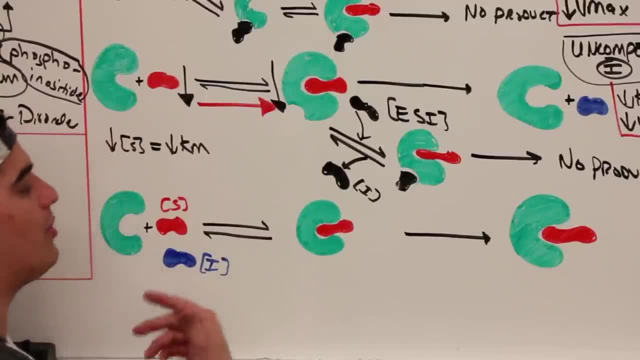 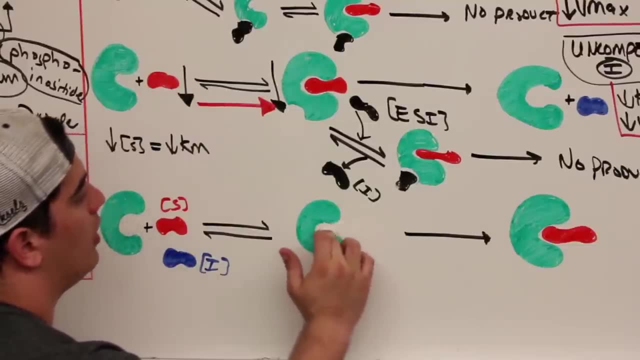 it's going to act kind of like a substrate, But it's going to perform what's called a substrate analog. So again, let me actually get this one out of here And let's replace this one with blue. So now he binds in here. 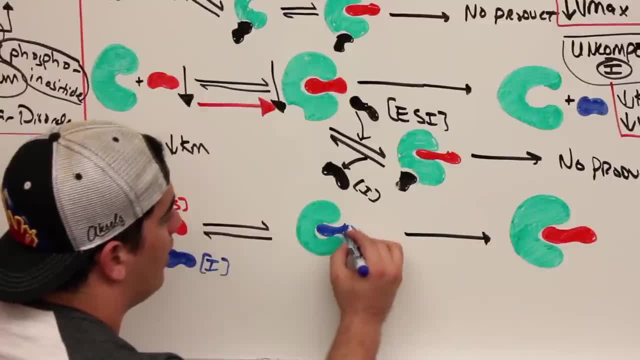 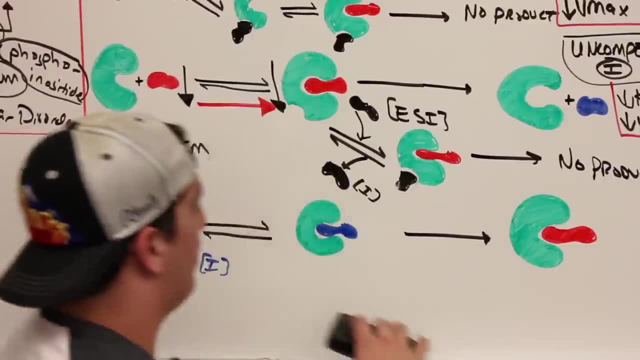 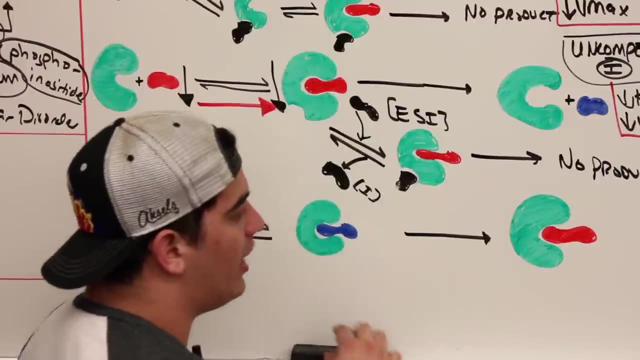 And when he binds in here he forms what's called a substrate analog. But here's where the bad thing happens: When this reaction occurs, this inhibitor right here, when it's bound into that active site. the difference between this and competitive inhibitors. 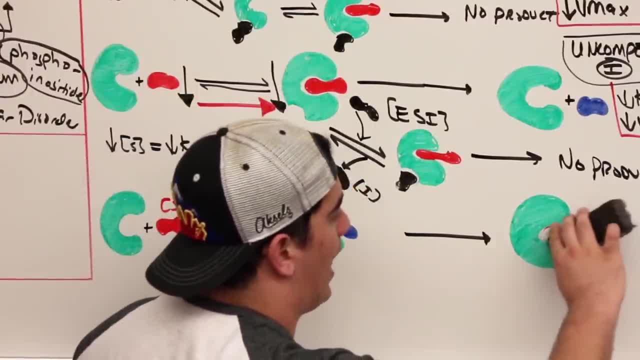 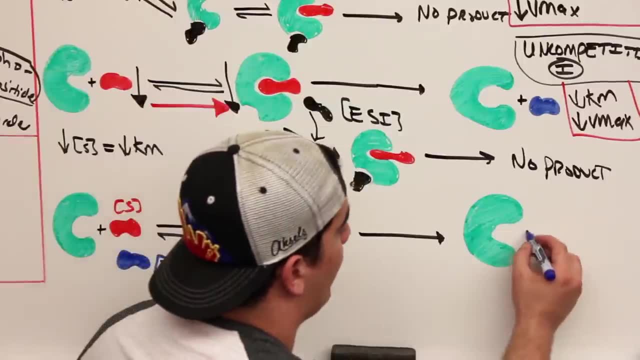 is the competitive inhibitors through weak interactions, weak bond interactions. But what happens with this one right here, this irreversible inhibitor, or what's called suicide inhibitor- and we'll talk about it- is that substrate analog forms what's called a covalent bond. 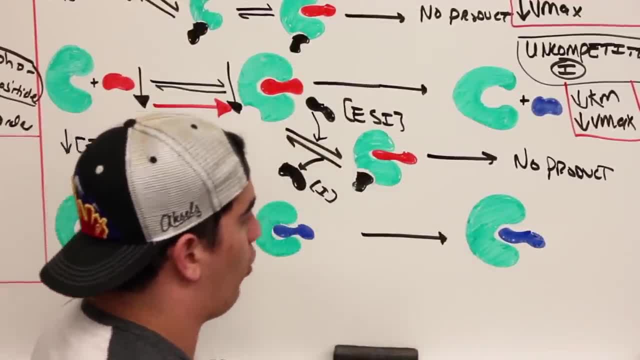 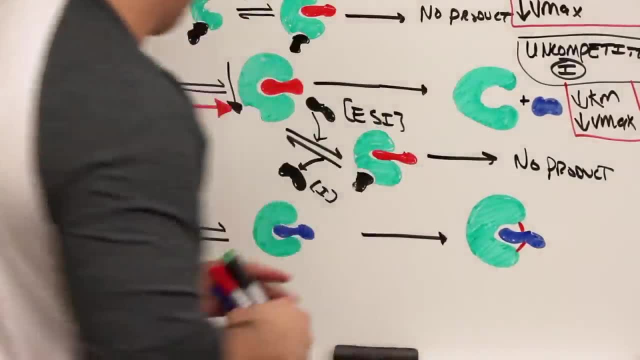 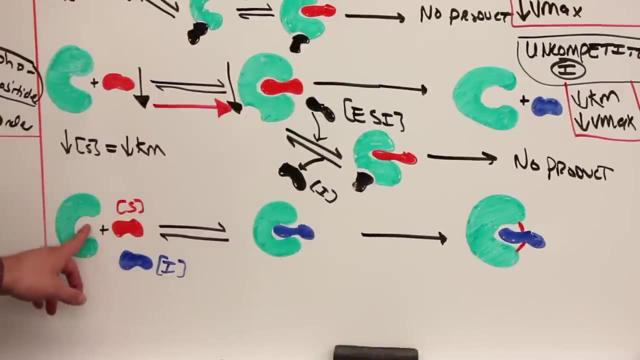 So I'm going to draw this covalent bond in red. So look here It forms what's called a covalent bond. So basically, what happens here? you have an enzyme. It likes to bind a normal substrate, But then this inhibitor binds into the active site and acts like a substrate analog. 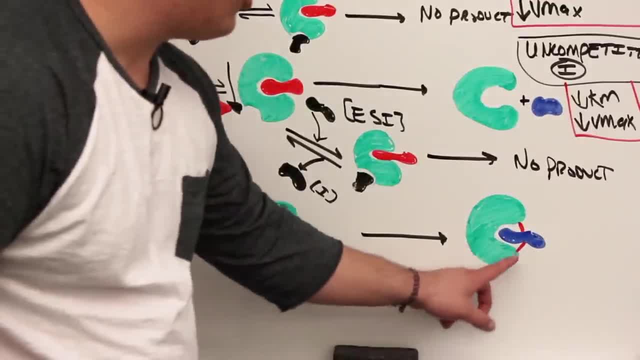 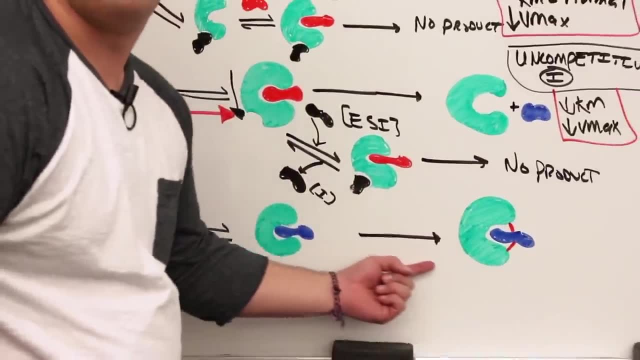 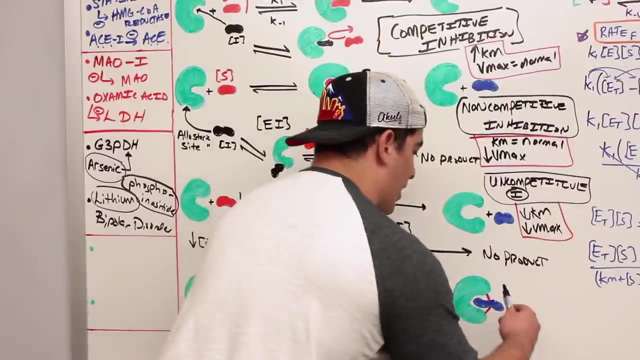 When it acts like a substrate analog, it forms what's called a covalent bond, which is a very strong bond. And then look what happens. Is this reaction reversible? No, So this enzyme is stuck in this form. And what is an example of this inhibition which is irreversible? 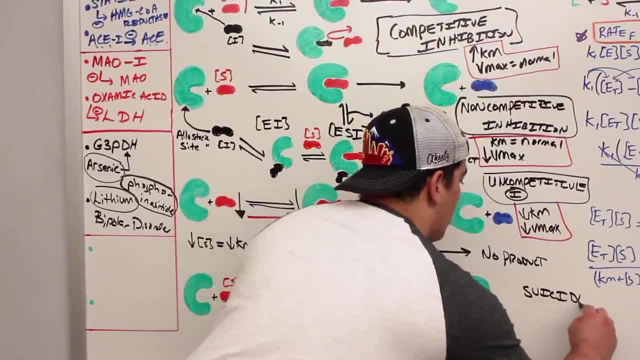 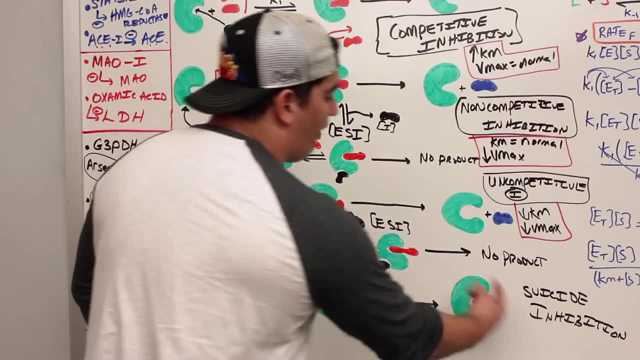 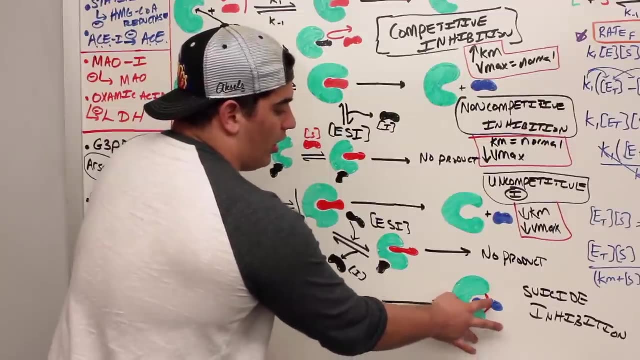 It's called suicide inhibition. Okay, So suicide inhibition, So it undergoes this covalent modification, in other words, And when it forms a covalent bond via this substrate analog with covalent bond to the enzyme. this is not reversible. 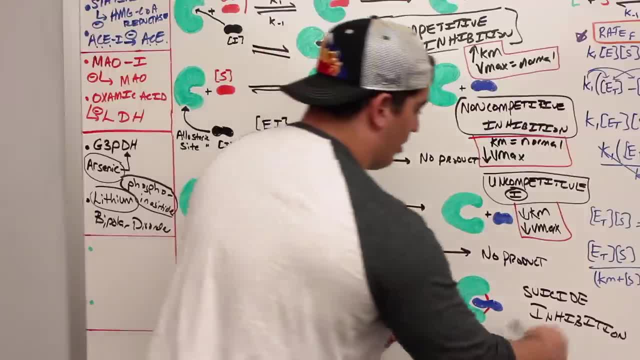 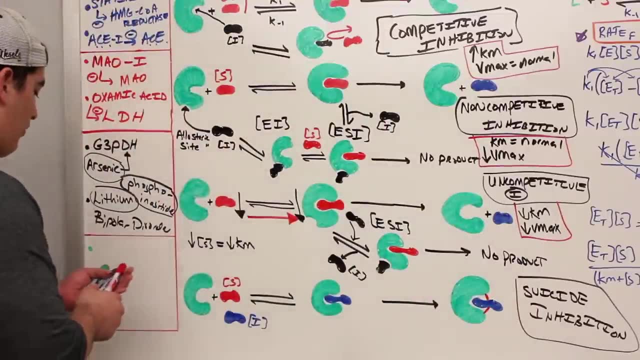 And this is very, very bad. Why So? again, this is suicide inhibition. These ones are super dangerous inhibitors. I'll give you an example of one of the worst ones, and we know it. You know it can be used in like certain types of chemical warfare, right? 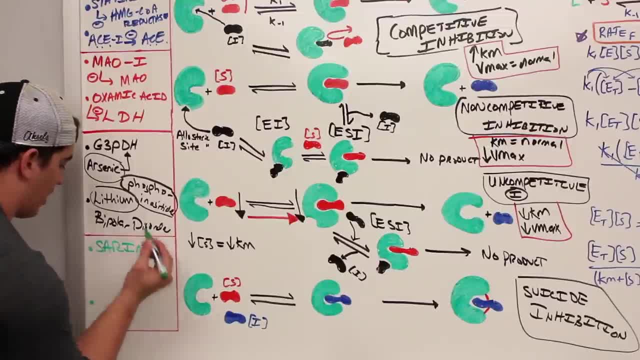 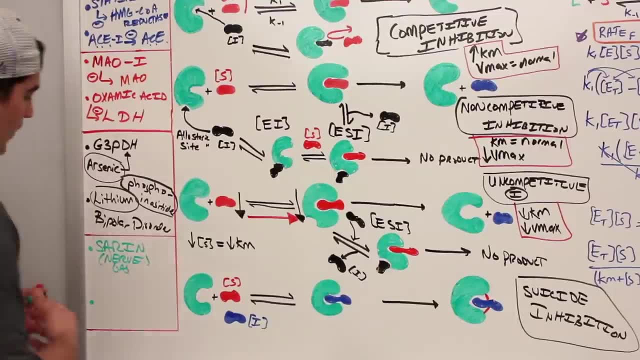 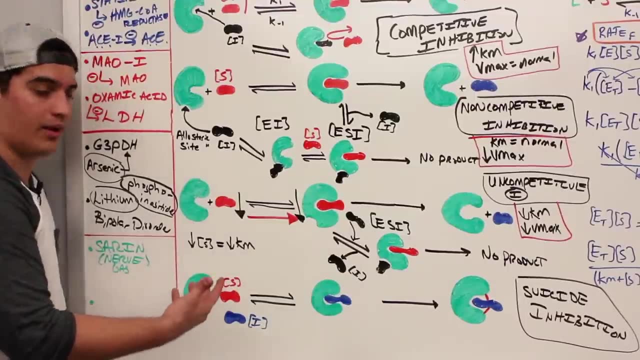 It's called sarin. So sarin is nerve gas And basically what this sarin does is- let's pretend, this enzyme is what's called acetylcholinesterase, which is normally responsible for breaking down acetylcholine. Well, if you give sarin, 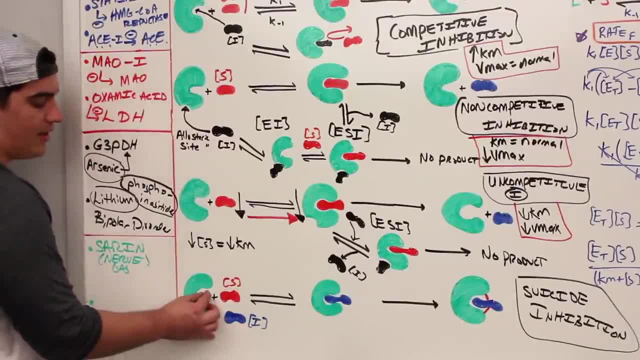 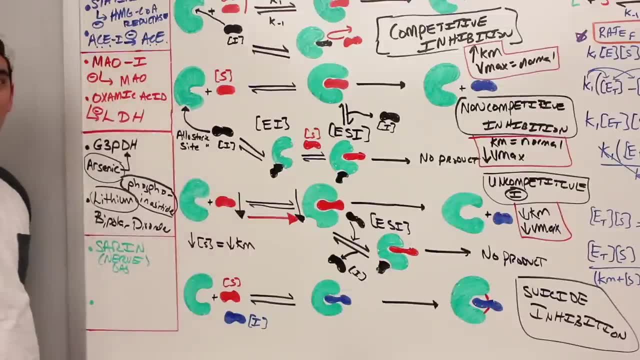 sarin's going to act as the inhibitor. It's going to bind in to this acetylcholinesterase, act as a substrate analog and then form a covalent bond with the acetylcholinesterase. And then what happens? 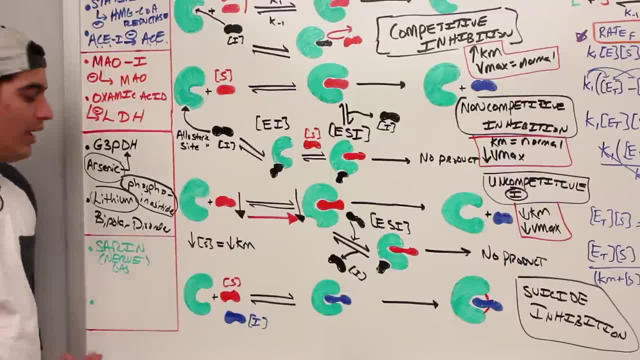 Can the acetylcholinesterase break down? the acetylcholine No, And these individuals die a very painful and quick death. Okay, So that's one example, Another one that's not a bad example. It can be actually. 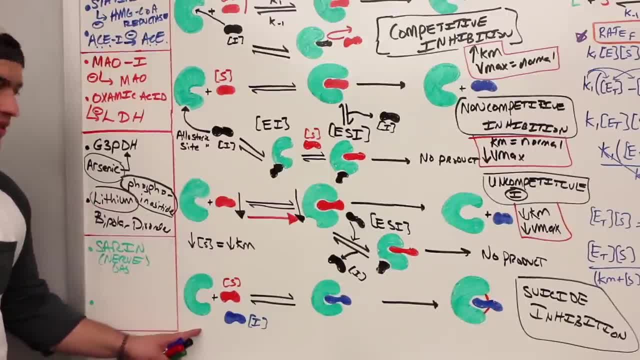 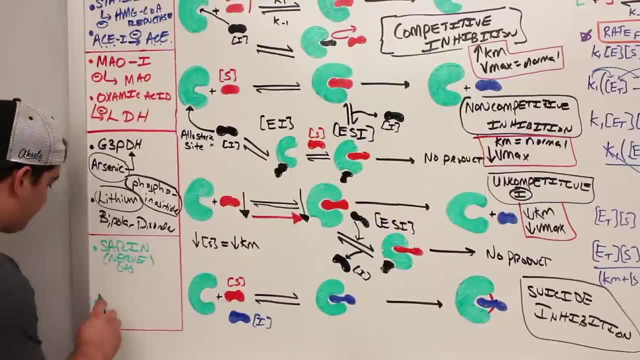 it's not always. it's not always bad. It depends on the specific you know, situation or physiological condition, But they also can be good. What's an example of a good one? Aspirin. Aspirin is a good example. 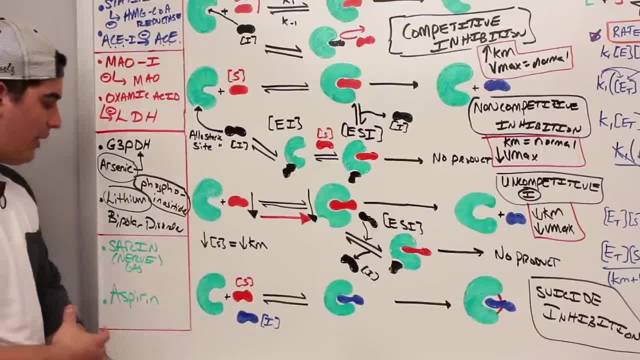 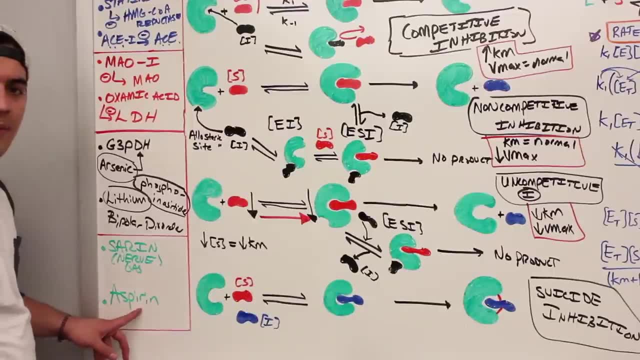 Because whenever you're having inflammation or certain types of blood clots and stuff like that, aspirin has the ability to inhibit certain types of enzymes. The enzymes are called cyclooxygenases. So what could be this enzyme? I'm going to put COX. 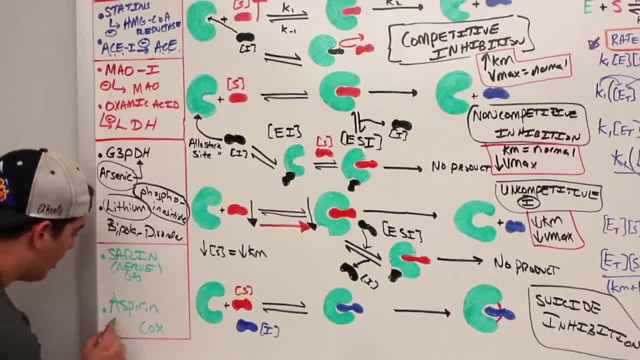 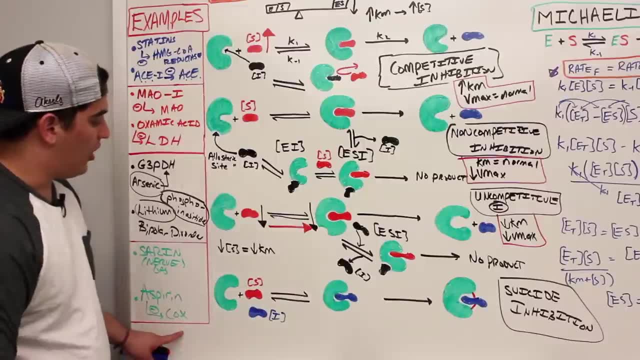 But remember, keep your minds clear. It's not what you think it is. And what does aspirin do? Aspirin can actually inhibit the cyclooxygenase enzymes. And again, how will it do it? Let's say that the normal substrate here for the cyclooxygenase 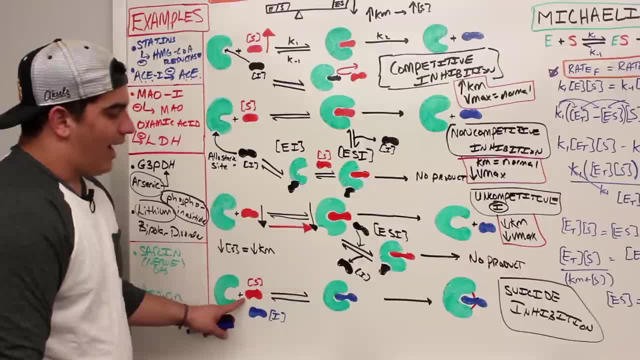 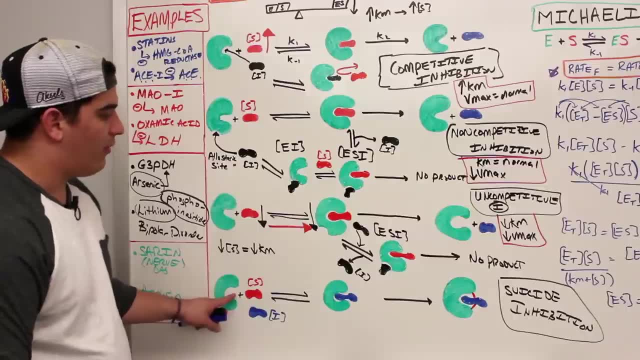 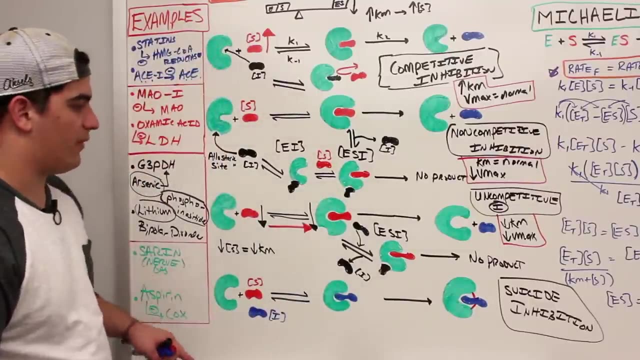 is going to be some type of basically arachidonic acid. What happens? The aspirin will actually come in, bind on to a specific enzyme and then form this actual covalent bond modification. Okay, So these are examples. these two are examples of what's called suicide inhibition. 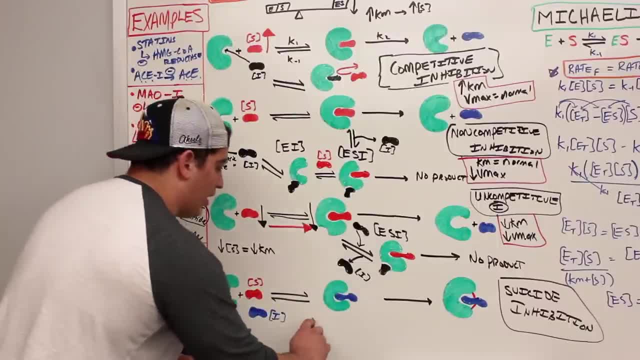 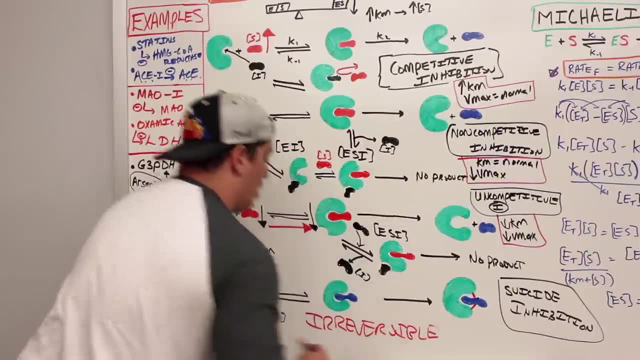 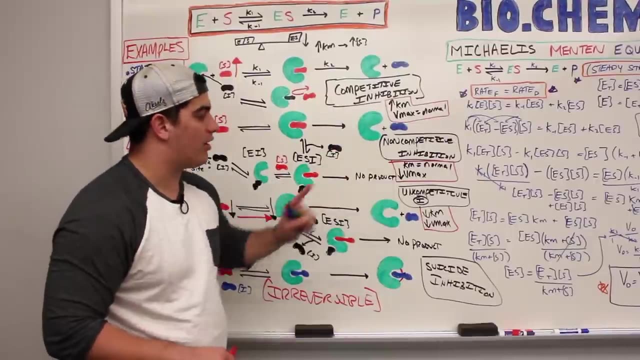 But, specifically, I need to make sure I write this completely clear: This is an irreversible inhibitor. Okay, This is irreversible inhibitors. These three that I talked about here- competitive, non-competitive, uncompetitive- are reversible inhibitors. Alright, guys, so in this video we talked about competitive.